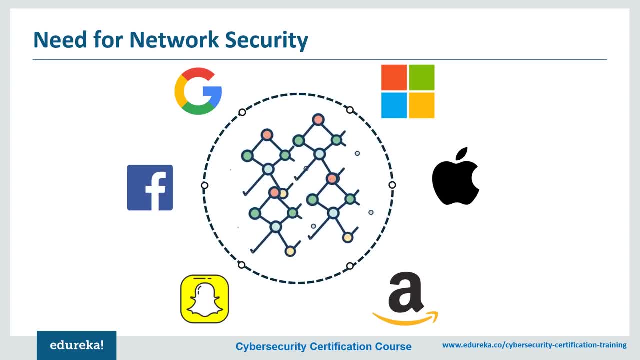 throughout the organization in an efficient and productive manner. organizational computer networks are now becoming a large and ubiquitous. assuming that each staff member has a dedicated workstation, a large-scale company would have few thousand workstations and many servers on the network. It is likely that these workstations may not be centrally. 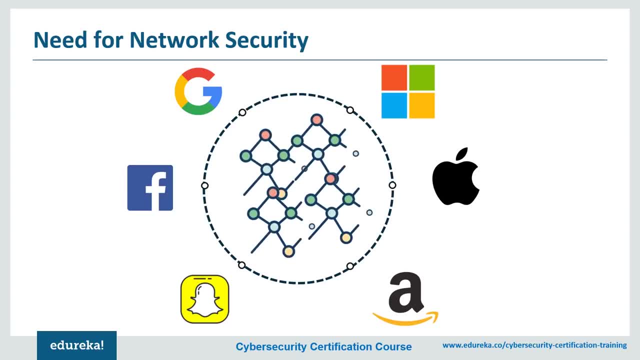 managed, nor would they have perimeter protection. now they have a variety of operating systems, Hardware, software and protocols with different level of cyber awareness among users. now imagine these thousands of workstations on company networks are directly connected to the internet. this order of unsecured Network becomes a target. 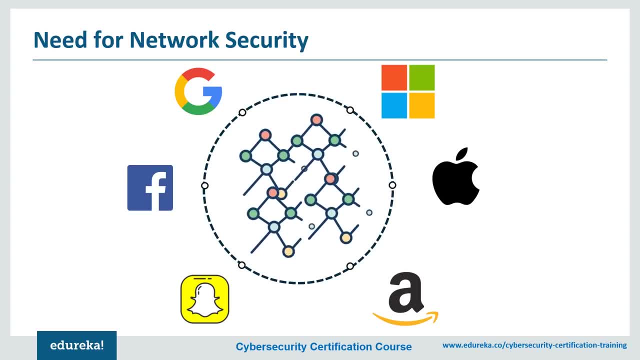 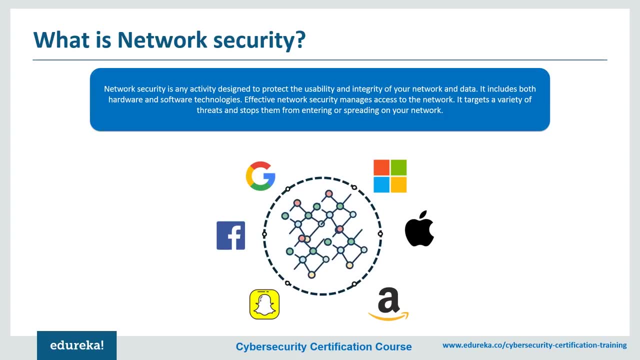 for an attack which holds valuable information and displays vulnerabilities. now, Network security consists of policies and practices adopted to prevent and monitor unauthorized access, misuse, modification or denial of a computer network and Network accessible resources. only Network security can protect you from a Trojan horse- viruses. Network security involves 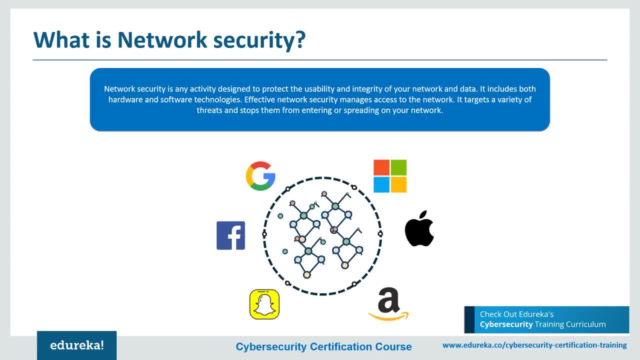 the authorization of access to data in a network which is controlled by the network administrator. users choose or are assigned an ID and password or other authenticating information that allows them to access to information and programs put in their authority. Network security covers transactions and communications among businesses, government agencies. 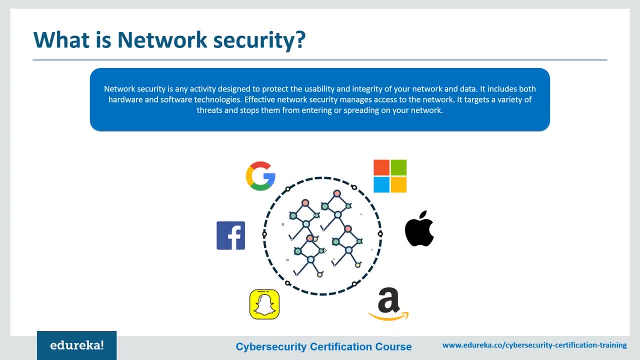 and individuals to networks can be private, such as within the company, and others which might be open to public access, and Network security is involved in organizations, enterprises and other types of institutions. It does as its title explains: it secures the network as well as protecting and overseeing operations being done. 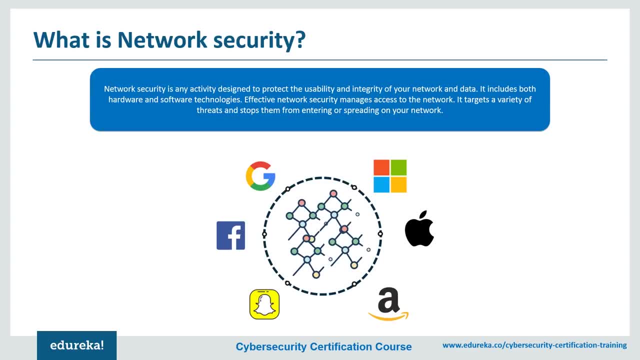 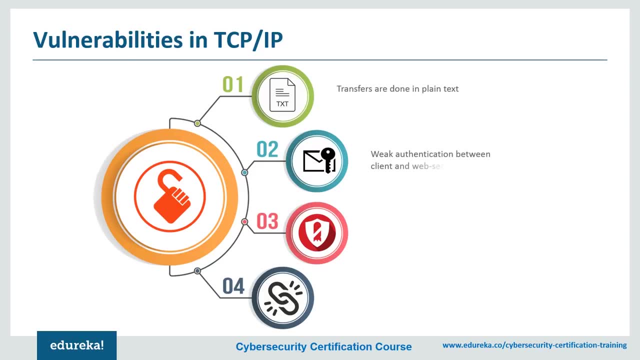 and the most common and simple way of protecting a network resource is by assigning it a unique name and a corresponding password. Okay, So now let's see why the need for Network security arose. So the TCP IP protocol suit, which is the major protocol suit, 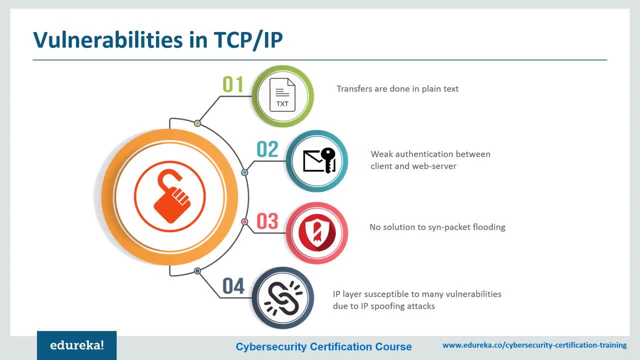 used for communication was created in 1980s as an internet working solution with very little concern for security aspects. It was developed for a communication in the limited trusted Network. However, over a period this protocol became the de facto standard for the unsecured internet communication. now some 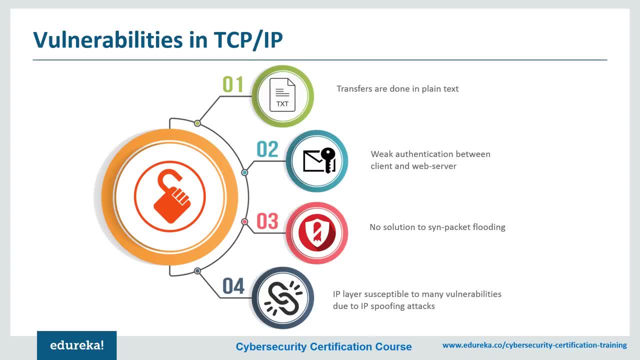 of the common security vulnerabilities of TCP IP protocol suits are as follows. Firstly, HTTP is an application layer protocol in TCP IP suit used for transfer files that make up the web pages for the web servers. These transfers are done in plain Network security for text. 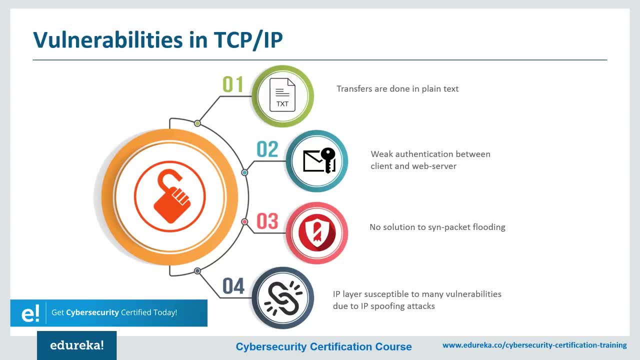 And an intruder can easily read the data packets exchanged between server and a client. another HTTP vulnerability is a weak authentication between the client and the web server during the initialization of the session. The vulnerability can lead to a session hijacking attack, where the attacker steals an HTTP session. 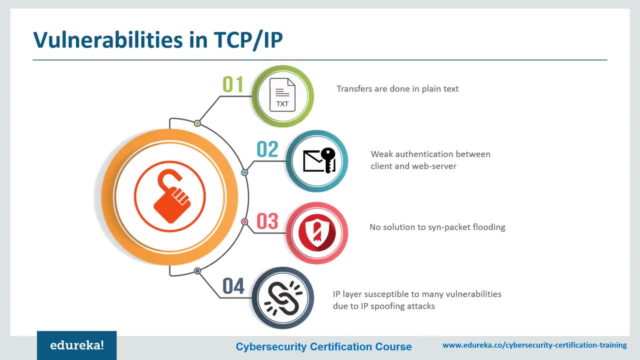 of the legitimate user. thirdly, TCP protocol vulnerability is the three-way handshake for connection establishment and attacker can launch a denial-of-service attack called sin flooding. to exploit this vulnerability, He establishes a lot of half-open sessions by not completing the handshake and this leads to server overloading and eventually a crash. 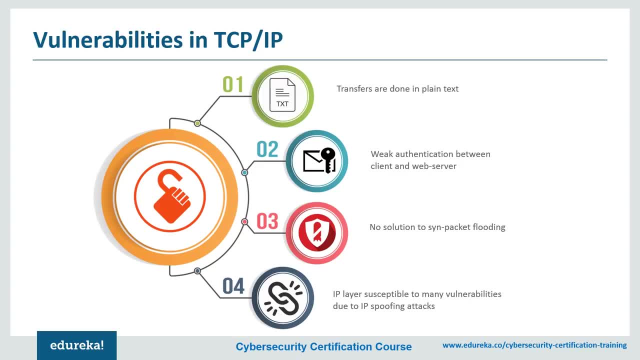 The fourth vulnerability is that the IP layer is susceptible to many vulnerabilities in itself through an IP protocol header modification and attacker can launch an IP spoofing attack that can be a serious conundrum to your business. now, apart from the four vulnerabilities mentioned, many other security vulnerabilities exist in TCP IP protocol family. 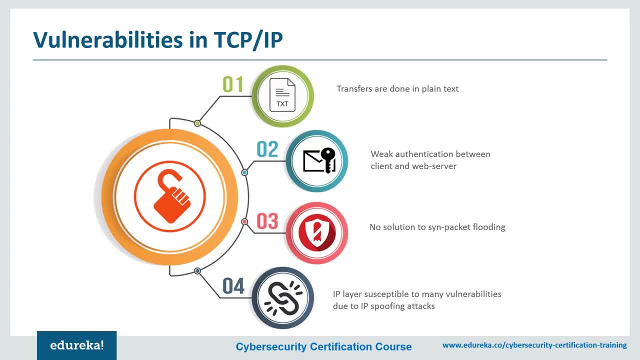 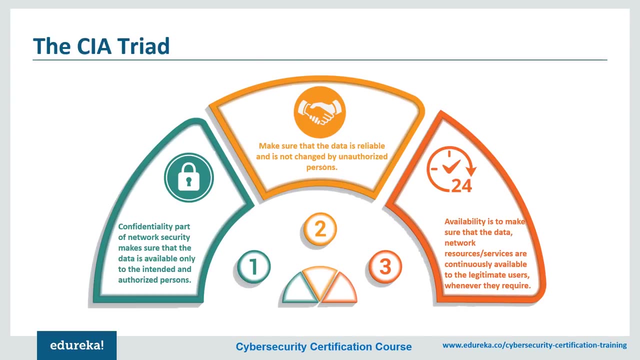 in design, as well in its implementation. incidentally, the IP based network communication. if one layer is hacked, the other layers do not become aware of the heart and the entire communication gets compromised. Hence there is need to employ security controls at each layer to ensure full proof security. now. 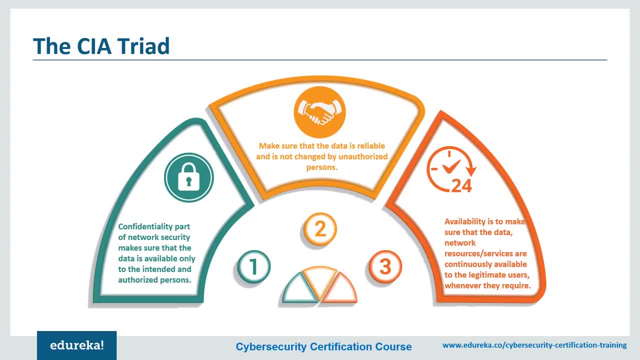 as discussed earlier, there exists large number of vulnerabilities in the network. thus, during transmission, data is highly vulnerable to attacks, and attacker can target the communication channel, obtain the data and read the same or reinsert a false message to achieve his nefarious aims. now Network security is not only concerned about the security. 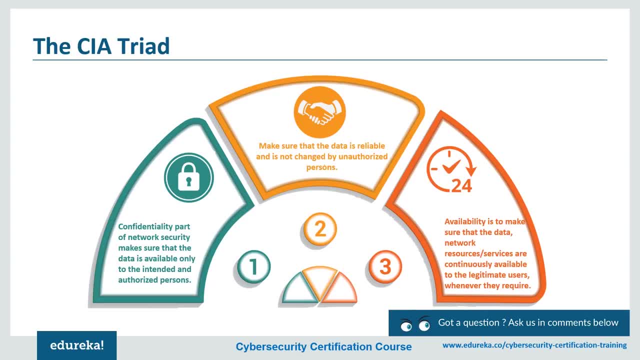 of the computer at each end of the communication chain. However, it aims to ensure that the entire network is secure. network security entails protecting the usability, reliability, integrity and safety of network and data effectively. now, network security defeats a variety of threats from entering or spreading on a network. 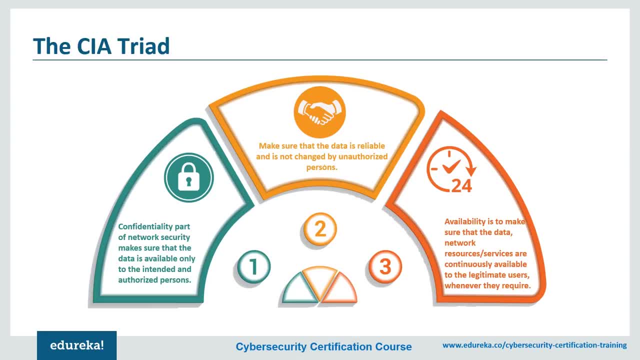 The primary goal of network security are confidentiality, integrity and availability. these three pillars of Network security are often represented as a CIA triangle. The function of confidentiality is to protect precious prisoners data from unauthorized person. confidentiality, part of Network security, makes sure that data is available only to the intended and authorized people. next the goal. 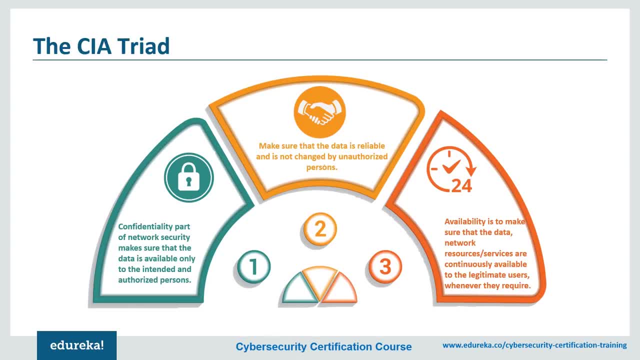 of integrity is the maintenance and assurance of accuracy and consistency of data. The functions of integrity is to make sure that data is reliable and is not changed by unauthorized people and, last but not the least, the function of availability and network security is to make sure that data network 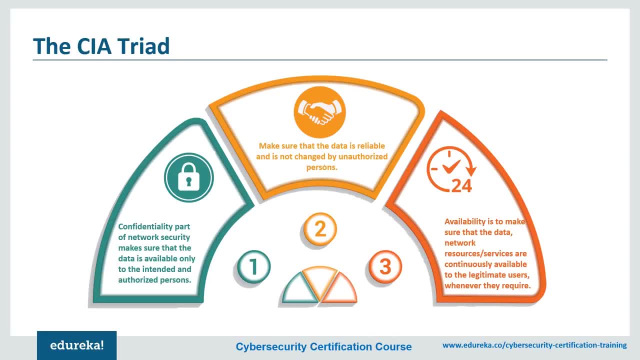 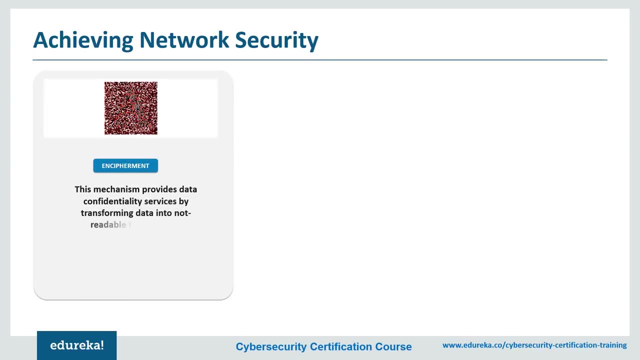 and its resources are continuously available to the legitimate user when they require it. now ensuring network security may appear to be very simple. the goals to be achieved seem to be straightforward, but in reality, the mechanism used to achieve these goals are highly complex, and understanding them involves sound reasoning. 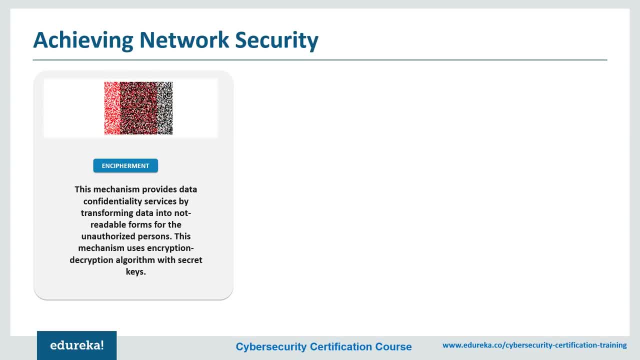 international telecommunication Union, or the ITU, and its recommendation on security architecture of x.8 00, has defined certain mechanisms to bring the standardization in methods to achieve Network security. some of these mechanisms are as encipherment, So this mechanism provides data confidentiality services. 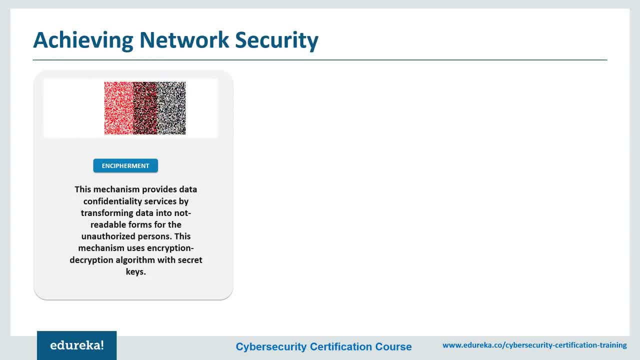 by transforming data into not readable forms for the unauthorized people. this mechanism uses encryption and decryption algorithm with the use of secret keys. next is digital signatures. Now, this mechanism is the electronic equivalent of ordinary signatures in electronic data. It provides authenticity of the data. third is access control. 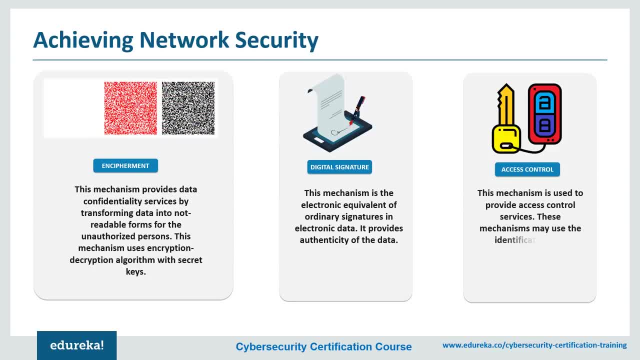 This mechanism is used to provide access control services. These mechanisms May use identification and authentication of an entity to determine and enforce the access rights of the entity before he touches anything on the network. now, having developed and identified various security mechanisms for achieving Network security, 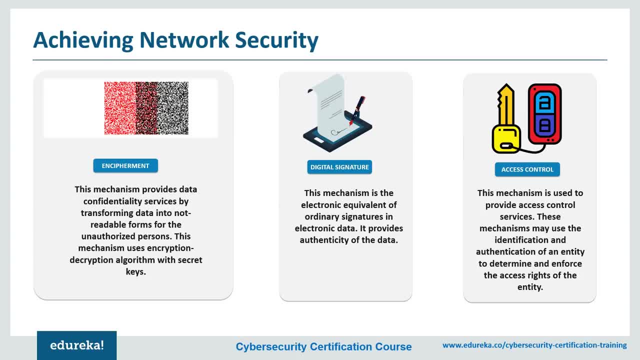 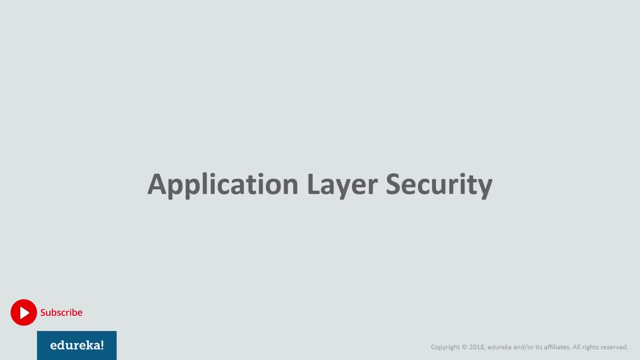 It is essential to decide where to apply them, both physically, at what location and, logically, at what layer of an architecture such as TCP, IP. Okay, so it's time we discuss the application layer security, and this is the first layer that we're going to discuss. 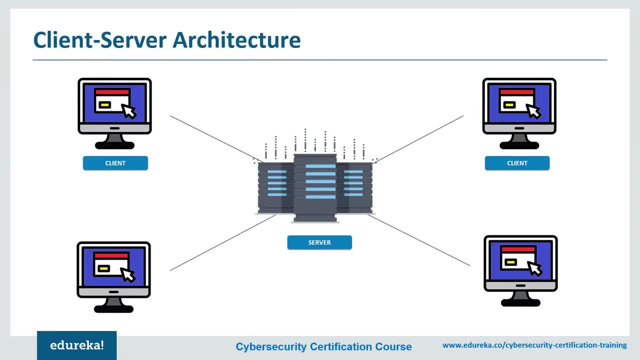 in today's tutorial. now, various business services Are now offered online through client server applications. The most popular form are web applications and email. in both applications, the client communicates to the designated server and obtain services. while using a service from any server application, the client and server exchange a lot of information. 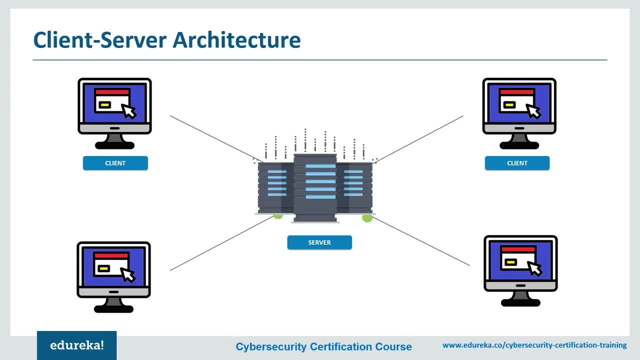 on the underlying internet and internet. We are aware of the fact that these information transactions are vulnerable to various attacks. now network security and tail securing data against attacks while it is in transit on a network. to achieve this goal, many real-time security protocols have been designed. such protocols need to provide: 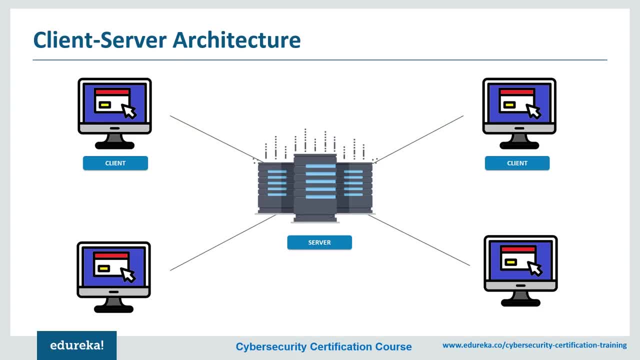 at least the following primary objectives: Firstly, the parties can negotiate interactively to authenticate each other. secondly, establish a secret session key before exchanging information on a network. and, last but not the least, the exchange information must be in encrypted form. Interestingly, these protocol work at different layers. 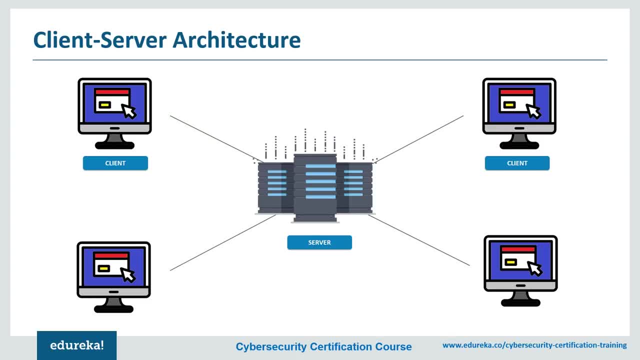 of networking model. For example, the s mime protocol works at an application layer and the SSL protocol is developed to work at the transport layer and the IP sec protocol works at the network. here. So we are going to discuss how email security works, because it's very important to the application layer security. 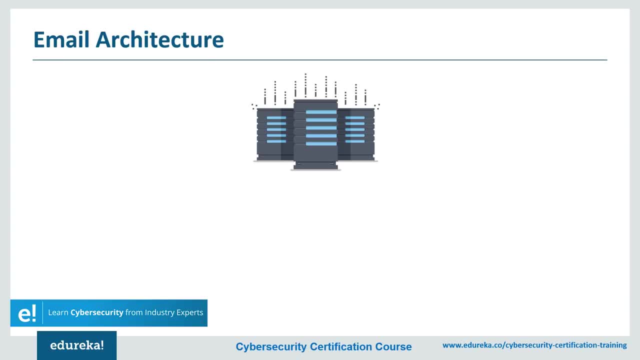 as many of the application layer, information is mostly through emails or web server architectures, We're going to choose email for this one Now. the simplest way of sending an email would be sending a message directly from the senders machine to the recipients machine, in this case. 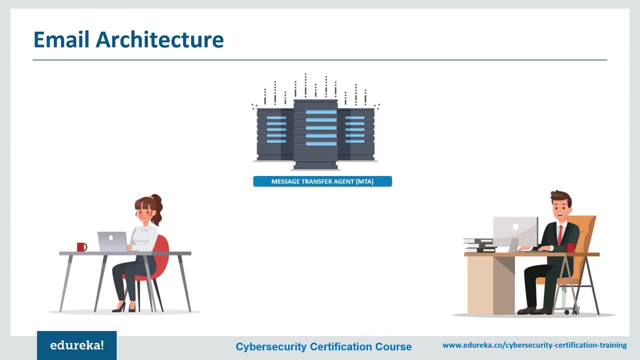 It is essential for both machines to be running on the network simultaneously. However, this setup is as impractical as users may occasionally connect to their machines to the network. Hence the concept of setting up email servers arrived in the setup. the mail is sent to the email server. 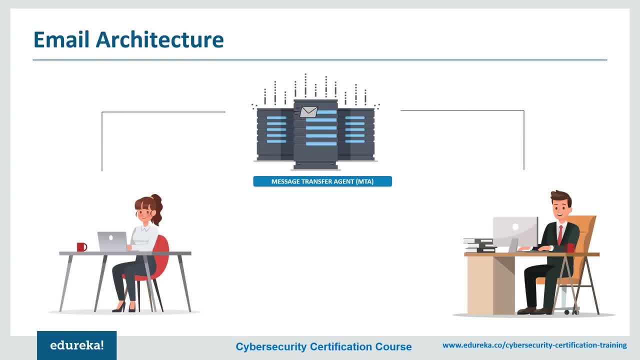 which is permanently available on the network. when the recipients machine connects to their network, It reads the mail from the mail server and, in general, the email infrastructure consists of a mesh of mail servers, also termed as a message transfer agent or an MTA, and the clients machines running. 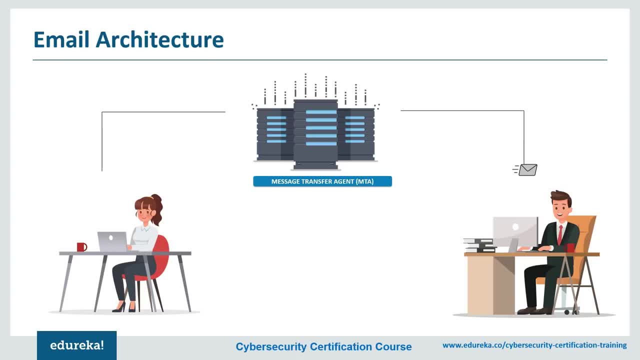 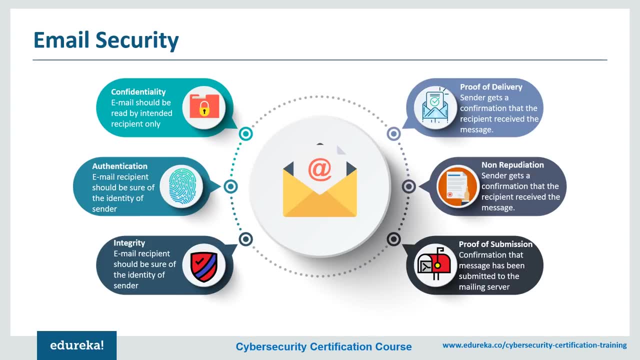 an email programming comprising of a user agent and a local MTA. Now, the growing use of email communication for important and crucial transactions demands provision of certain fundamental security services, such as the following: firstly is confidentiality: now email messages should not be read by anyone but the intended recipient. second is authentication. 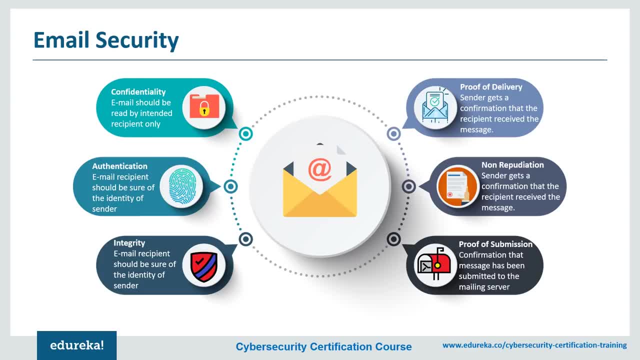 that is, email recipient can be sure of the identity of the user. third is integrity, and that is assurance to the recipient that the email message has not been altered since it was transmitted by the sender. next is proof of delivery, that is, the sender gets a confirmation. 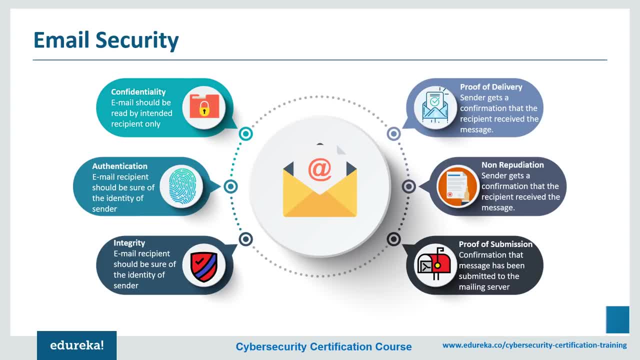 That the recipient received the message. second last is non-repudiation, which is email recipient is able to prove to a third party that the center really did send the message. Lastly, we have proof of submission, which is that the email sender gets confirmation. 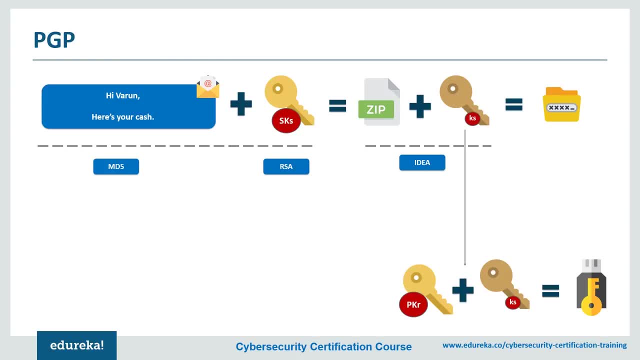 that the message is handed over to the mail delivery system. now, security services such as privacy, authentication, message Integrity and non-repudiation are usually provided by using public key cryptography. now pretty good. privacy or PGP is an email encryption scheme. It has become the de facto standard. 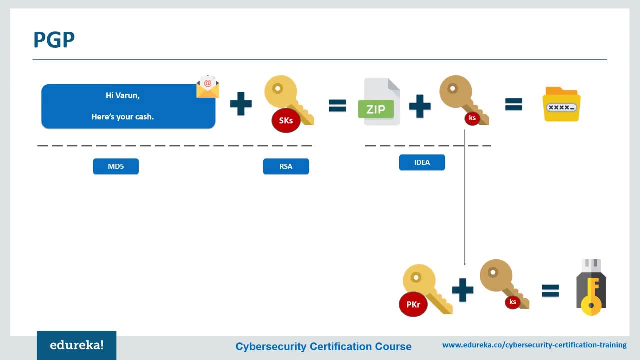 for providing security services for email communication. now, as discussed, it uses public key cryptography, symmetric key cryptography, hash functions and digital signatures. It provides privacy, sender authentication, message Integrity and non-repudiation. now, along with these security services, It also provides data compression and key management support PGP uses. 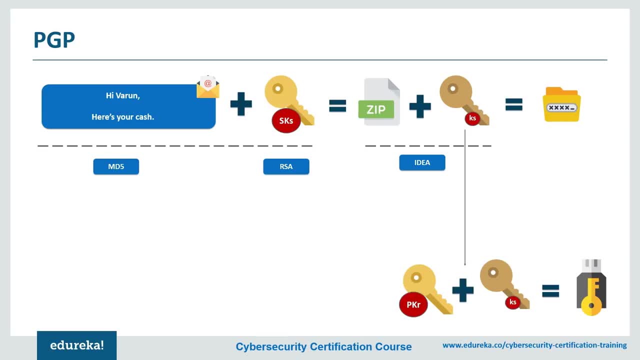 existing cryptographic algorithms, such as RSA, IDEA, MD 5, Etc. rather than inventing the new one. So how does PGP exactly work? Well, firstly, we have a message. for example, Hi Varun has your cash. So now this message is hashed using the MD 5 algorithm. 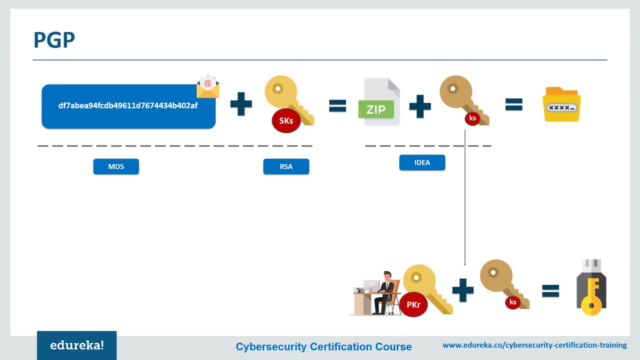 and a hash is actually made. now the result in 128-bit hash is signed using the private key of the sender using the RSA algorithm. Next, the digital signature is concatenated to the message and the result is compressed. now 128-bit symmetric key KS, is generated and used to encrypt the compressed message. 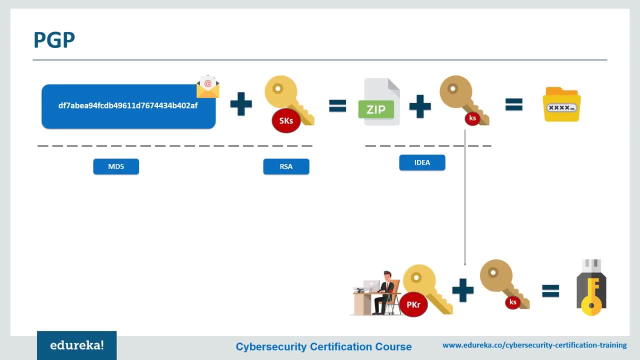 with the International data encryption algorithm, or IDEA. Now the symmetric key, KS, is encrypted using public key of the recipient using RSA algorithm, and the result is appended to the encrypted message. Now PGP key certificate is normally established through a chain of trust. For example, is public key is signed by P using his public key. 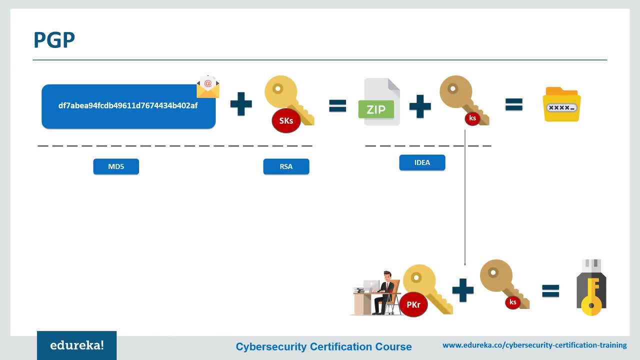 and beast public key is signed by C using his public key. as this process goes on, it establishes a web of trust in a PGP environment. any user can act as a certifying Authority and any PGP user can certify another PGP users public key. 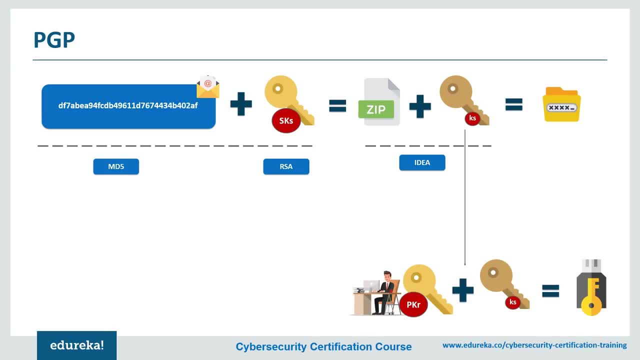 However, such a certificate is only valid to another user if the user recognizes the certified as a trusted introducer. several issues exist with such a certification method and it may be difficult to find a chain leading from a known and trusted public key to desired key. 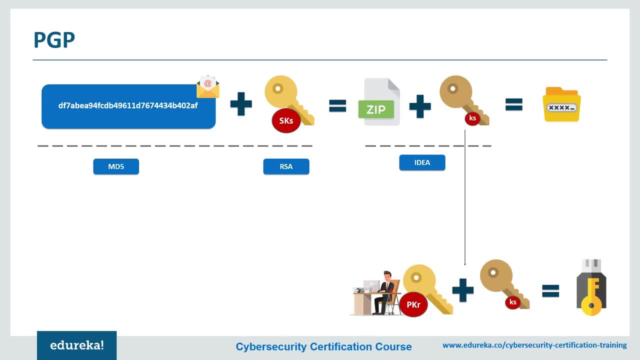 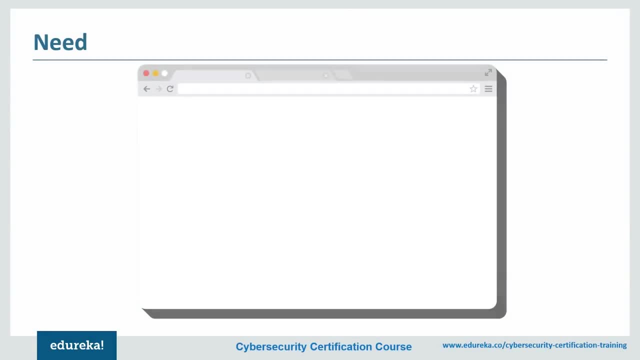 Also, there might be multiple chains, which can lead to different keys for desired users. Okay, so that was all about application layer security. It's time We move to the transport Leo now. So suppose you're visiting a shopping site like jabongcom. 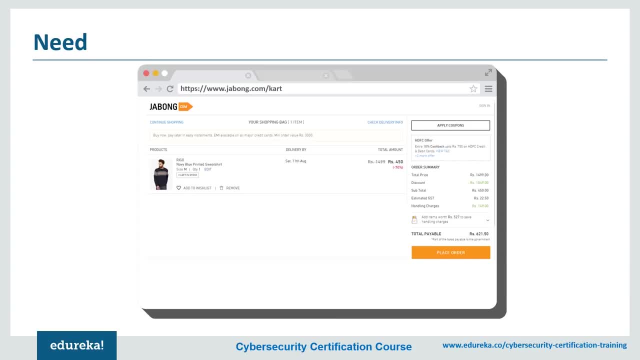 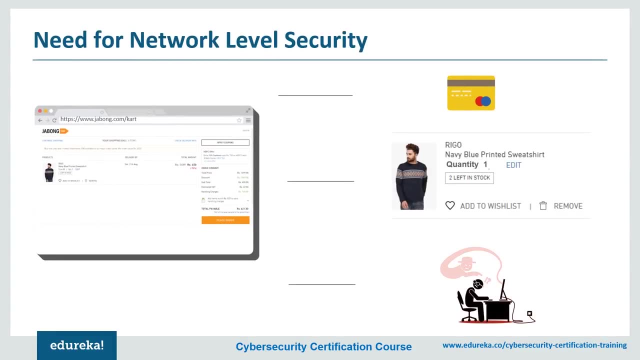 and you want to buy a sweatshirt. Now you enter the type of good and the quantity desired, and then the address and payment card details. Now you click on submit and wait for the delivery of goods with debit price of amount from the account. Now all this sounds good. 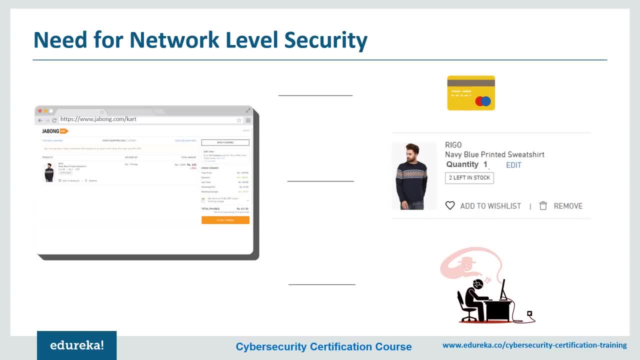 but in the absence of network security, you could face a few surprises. For example, if the transaction did not use confidentiality and attacker could obtain your payment card information, and then the attacker can then make purchases at your expense. if no data Integrity was used in the communication and attacker could modify Bob's order. 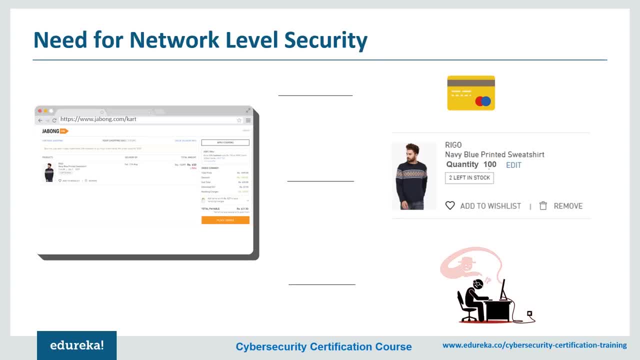 in terms of type or quantity of goods. Lastly, if no server authentication was used, a server could display the website and its famous logo, but the site could be malicious site maintained by an attacker who's masquerading as jabongcom. and after receiving your order. 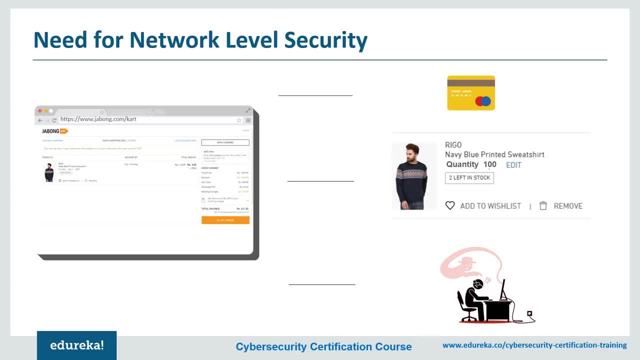 he would take your money and flee, or he could carry out an identity theft by collecting all your name and your credit card details. now, transport layer security schemes can address these problems by enhancing TCP, IP based network communications with confidentiality, data Integrity, server authentication and client authentication: the security at the Slayer. 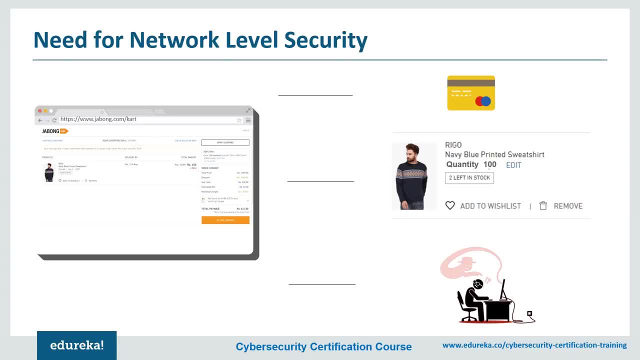 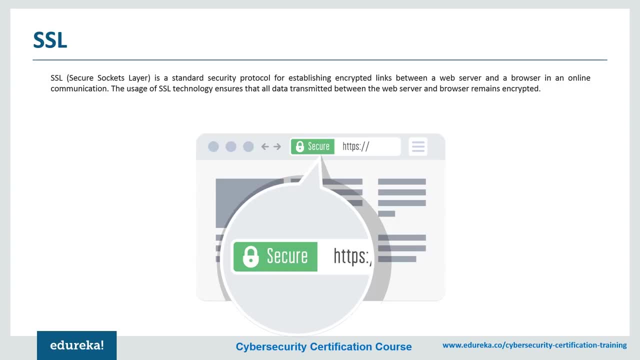 is mostly used to secure HTTP based web transactions on a network, and this is mostly done through a protocol called SSL. Okay, so in the year 1995 Netscape developed SSL version 2 and is used in Netscape Navigator 1.1.. 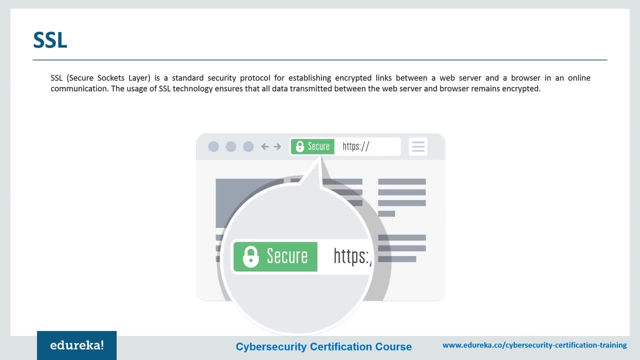 The SSL version 1 was never published and used. later, Microsoft improved upon SSL version 2 and introduced another similar protocol named private communication technology or PCT. Netscape substantially improved SSL version 2 on various security issues and then deployed SSL version 3 in 1999.. 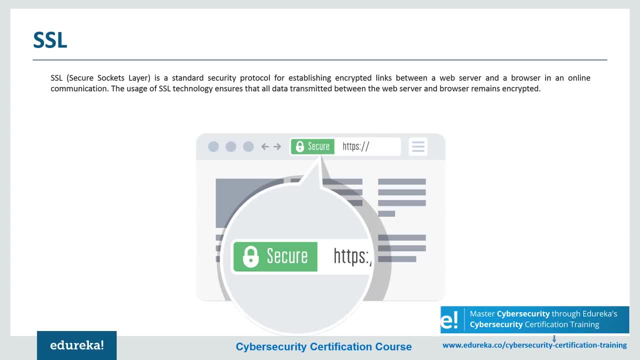 The internet engineering Task Force subsequently introduced a similar TLS protocol. as an open standard, TLS protocol is non-interoperable with SSL version 3. now, TLS modified the cryptographic algorithms for key expansion and authentication. also, TLS suggested use of open crypto, RFE, Hellman and digital signature standards in place. 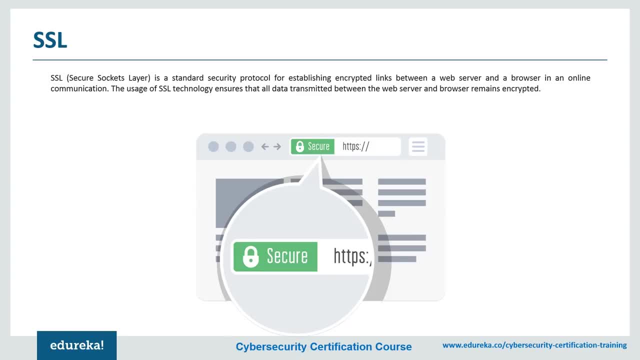 of patented RSA that is used in SSL. but due to the expiry of RSA patent in 2000, there existed no strong reason for users to shift away from the widely deployed TLS to SSL version 3.. So this is why SSL version 3 is mainly used over TLS. 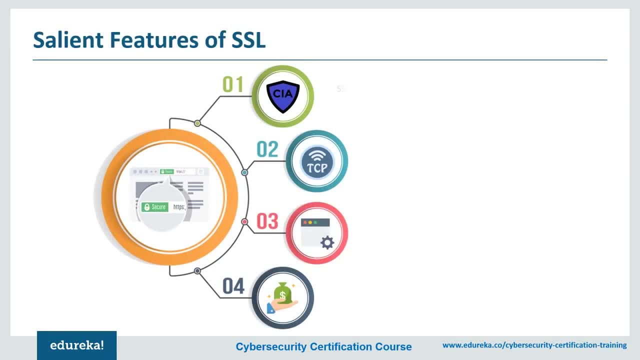 in various sites and applications. So the silent features of SSL protocol are as follows: as a still provide network connection security through confidentiality, that is, information is exchanged in an encrypted form. then it provides authentication, Which is communication entities identify each other to the use of a digital certificates web server authentication. 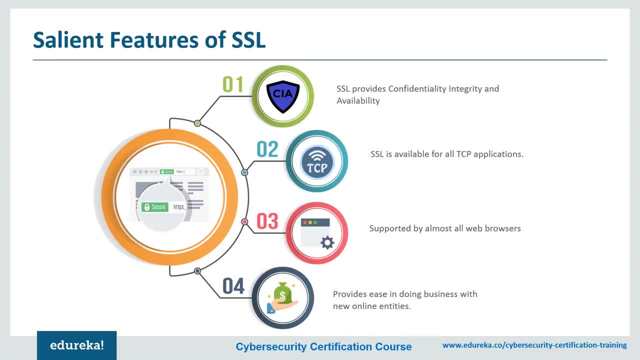 is mandatory, whereas client authentication is kept optimal. and third is reliability, which maintains message Integrity in check. moving on, SSL is always available for TCP applications and it is supported by almost all the web browsers. It provides ease and doing business with new online entities and is developed primarily for web e-commerce services. 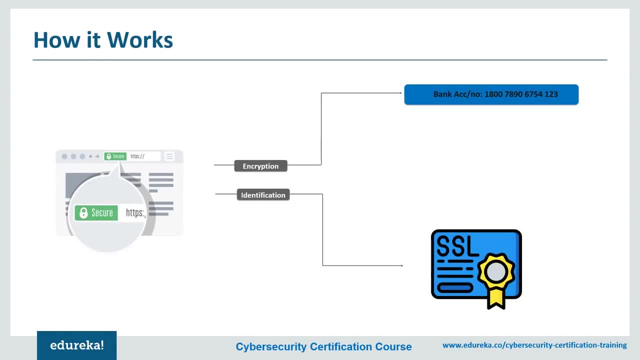 So how does SSL exactly work? Well, it does it in two ways. Firstly is by providing encryption and second identification. So suppose you were transferring a bank account number through some SSL and enabled website, then your bank account would be first encrypted and then the message would be transferred. 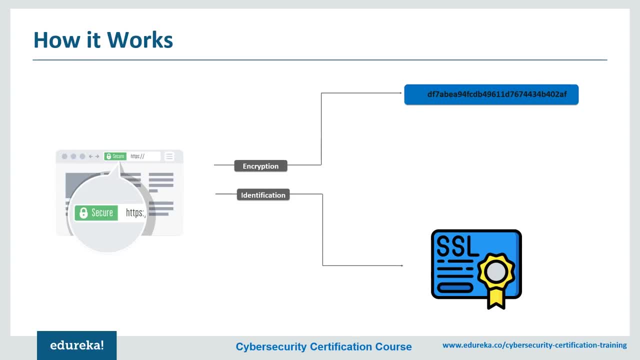 Secondly, identification is done using SSL with the help of SSL certificates. SSL certificates are small data files that are digitally bind a cryptographic key to an organization's detail. when installed on a web server, It activates the padlock and the HTTPS protocol and allows secure connection from a web server to a browser, typically SSL. 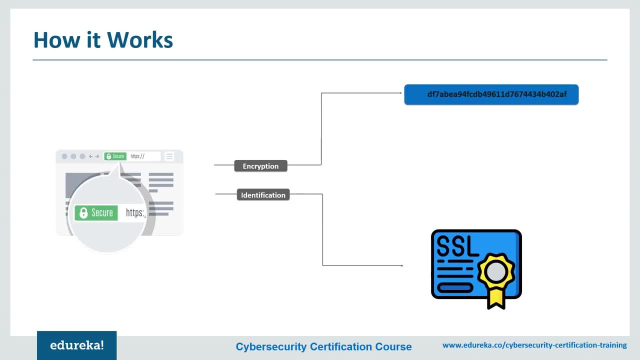 is used to secure credit card transactions, data transfers and logins and, more recently, is becoming the norm when securing browsing of social media sites. Now the SSL certificates binds together a domain name, a server or a host name, and an organization's identity is known by the certificate. 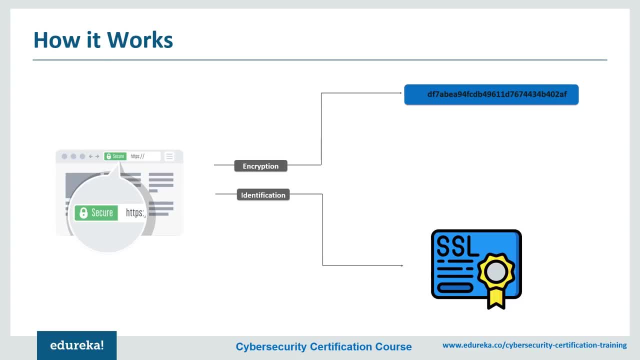 when he is on the web. So, when a website is using HTTPS, you know it's using HTTP, with the secure part provided by SSL That is provided by the SSL security certificates. Okay, so it's time we move to the most important layer. 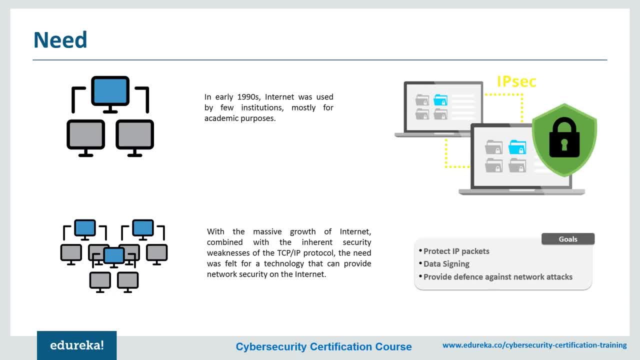 that is, the network layer security. now, in the early 90s internet was used by a few institutions, mostly for academic purposes. but in latter decades the growth of internet became exponential due to expansion of Network and several organizations using it for communication and other purposes. with the massive growth of internet combined, 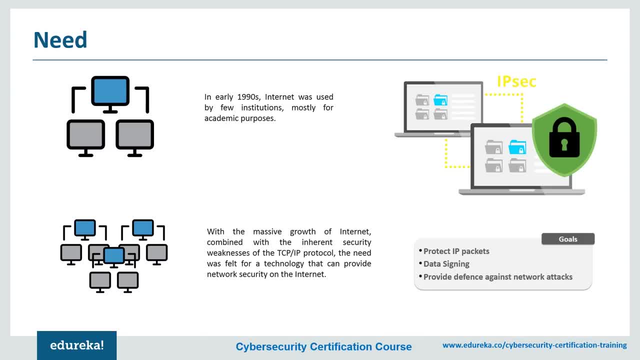 with the inherent security weakness of the TCP IP protocol, The need was felt for a technology that can provide Network security on the internet. a report entitled security in the internet architecture was issued by the internet architecture board in 1994.. It identified the key areas for security mechanisms. 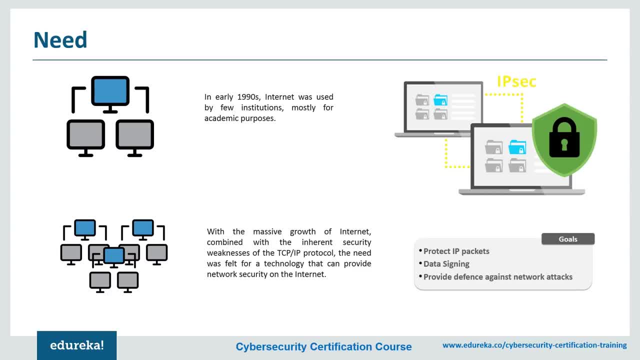 and the IAB included authentication and encryption as an essential feature in the IPv6, which is the next-generation IP. Fortunately, these security capabilities were defined such as they can be implemented with both the current IPv4 and futuristic IPv6. security frameworks include IP sec and has been defined. 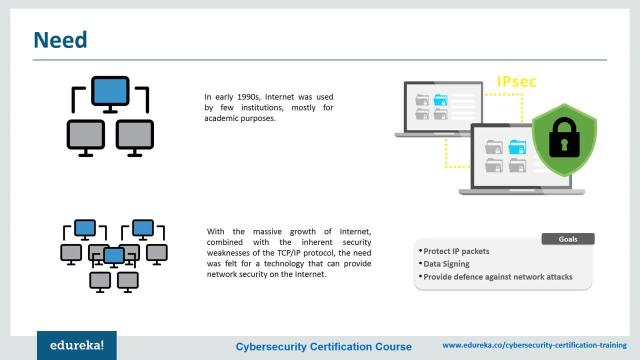 in several requests for comments, and some RFCs specify some portions of the protocol, while others address the solution as a whole. So the basic goals of IP sec, which is the protocol used for network security, is to protect IP packets, provide data signing and provide defense against network attacks. 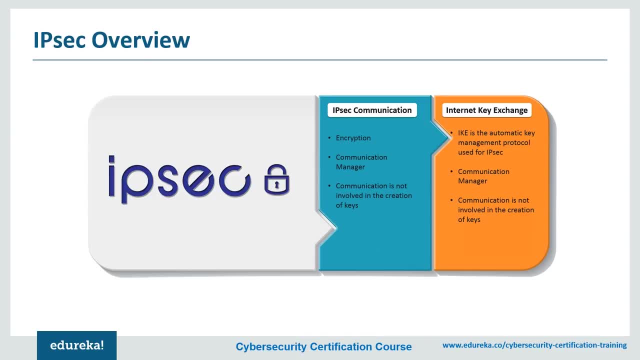 Okay, so let me give you guys an overview of IP sec before we continue. So the IP sec has two parts. first is IP sec communication and the second is internet key exchange. now, IP sec communication is typically associated with standard IP sec functionality. It involves encapsulation, encryption and hashing. 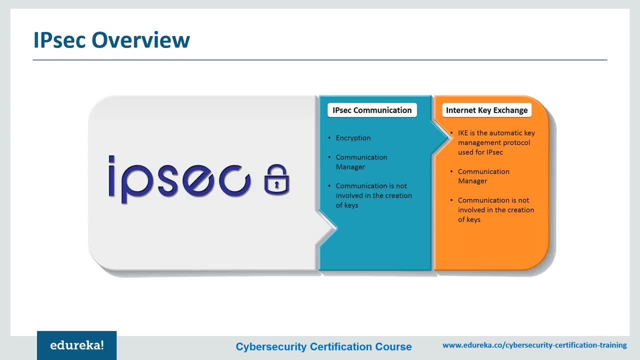 the IP datagrams and handling all IP packet processes. Secondly, it is responsible for managing the communication according to the available security associations established between communicating parties. next, it uses security protocols, just authentication header and encapsulated SP. It is also important to note that the IP sec communication is not involved. 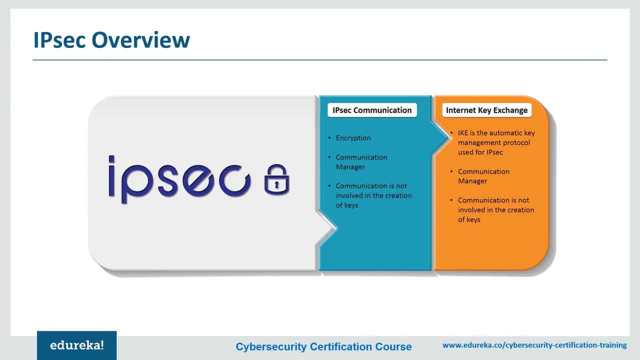 in the creation of keys or their management, and IP sec Communication operations itself is commonly referred to as IP sec. the second part of the IP sec protocol is the internet key exchange. internet key exchange is automatic key management protocol used for IP sec. technically, key management is not essential. 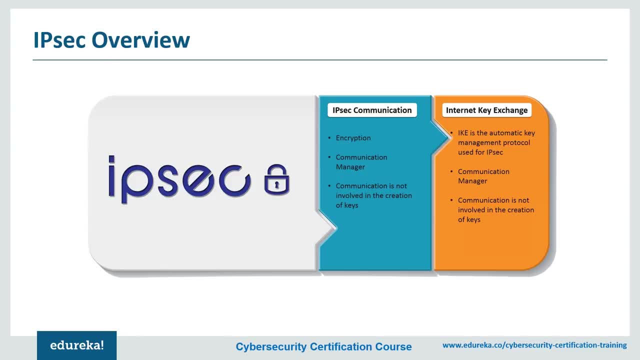 for IP sec communication, and the keys can be manually managed. However, manual key management is not desirable for large networks. thirdly, internet key exchange is responsible for creation of keys for IP sec and providing authentication during key establishment process, though, So IP sec can be used. 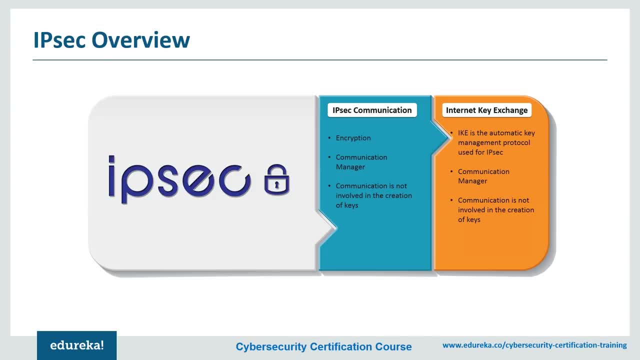 for any other key management protocols. Ike is used by default also for Ike defines two protocols called Oakley and SK EME to be used with already defined key management frameworks in Internet Security Association key management protocol. Okay, so let's just see how IP sec works. 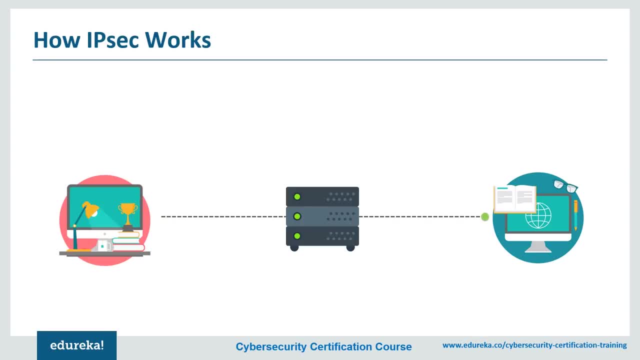 So, firstly, when two computers realize that they need to share data amongst themselves, They ask themselves one question, which is: will IP sec be used by the sending and receiving computers? now, if the answer to the question is yes, a security negotiation is actually established in the security negotiation and encryption algorithm. 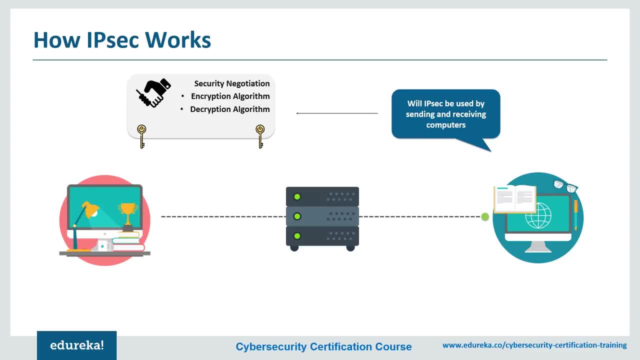 and decryption algorithm is discussed between the two computers that can be used for the exchange of data. now, during the security negotiation, a session key is also generated. now, after the security negotiation takes place, The session keys are actually made known to the two computers that are trying to communicate. 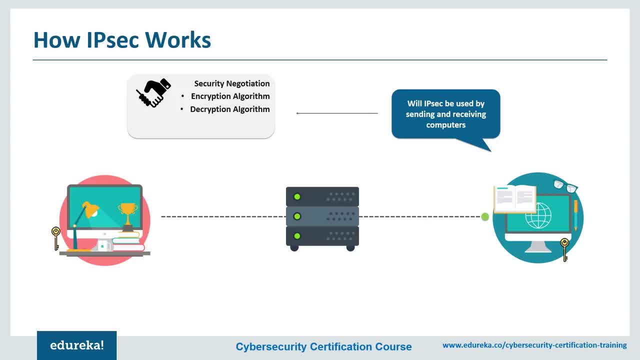 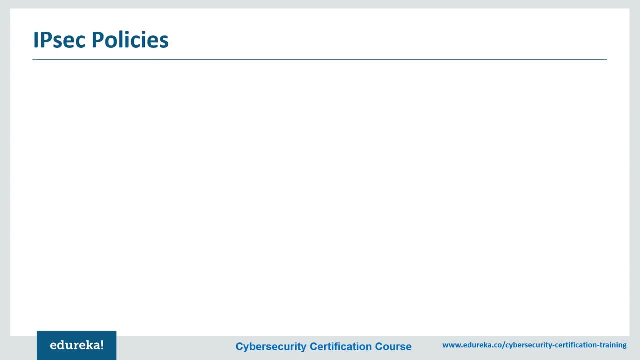 with each other, and they use these session keys for encryption and decryption purposes for the data That is being sent over the network now. So this is how IP sec works. now IP sec also consists of various policies that make it the de facto for network security protocols. 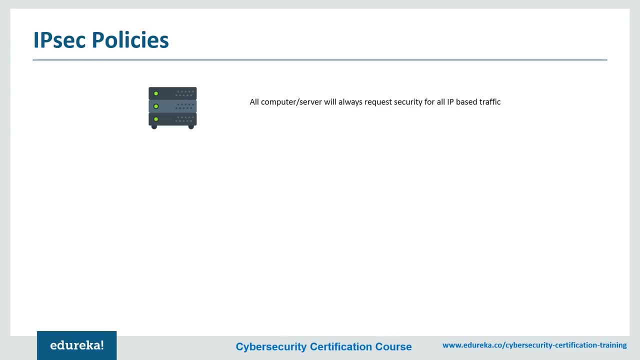 Now the first policy on the list is server request security policy. contrary to the name, this policy can be used on both clients and server PCs. This PC will use IP sec security for all outbound security, and this policy will accept insecure inbound communications. Now, if a client requests a secure session, the policy will allow. 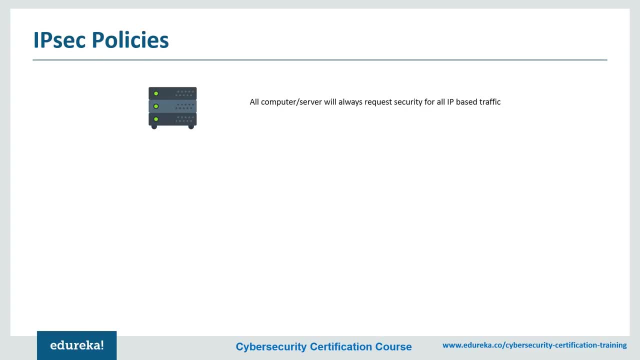 the client to establish one, which basically means that all computers and servers will always request for security for all IP based traffic. The second policy we have is client respond only policy. Now, this policy is designed to be run on client machines that don't normally need to worry about security. 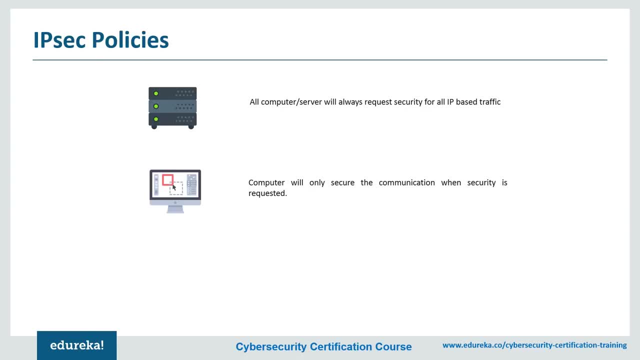 The policy is designed in such a way that the client will never initiate secure communication on its own. However, if a several requests that the client go into secure communication mode, the client will respond appropriately. now This means that computer will only secure the communication when the security 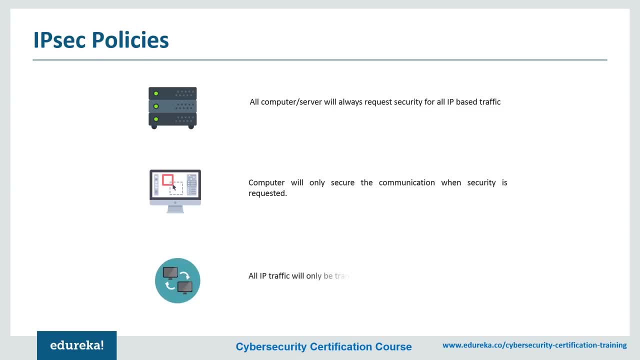 has been requested by the other person too. Now, the last policy of IP sec is the secure server or require security policy. now, according to this policy, all IP traffic that happened over a network will only be transferred over a secure connection. Okay, so that was all about security at the network, Leo. 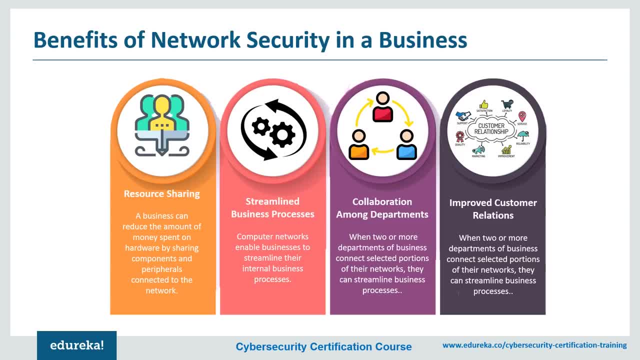 Now let's discuss the benefits of network security in a business. Nowadays, computer networks are viewed as a resource by almost all businesses. This resource enables them to gather, analyze, organize and this emirate information that is essential to their profitability. Most businesses have installed networks to remain competitive. 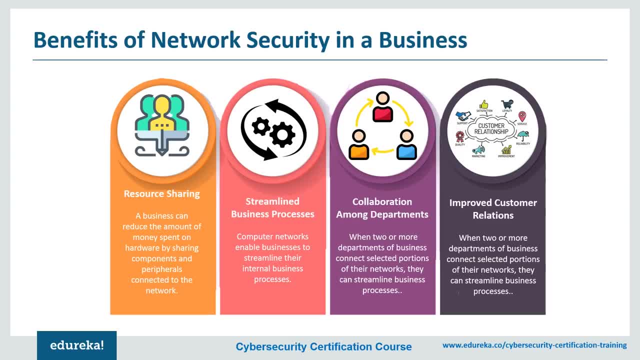 and the most obvious role of computer networking is that organization can store virtually any kind of information at the central location and retrieve it at desired place through the network. now benefits of computer networking: enables people to share information and ideas easily so they can work more efficiently and productively. networks improve activities. 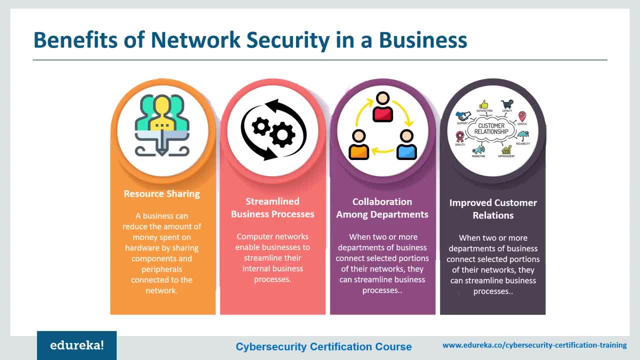 such as purchasing, selling and customer service. networking makes traditional business processes more efficient and more manageable And less expensive. now, the major benefits that a business draws from computer networks are as follows. firstly is resource sharing. a business can reduce the amount of money spent on hardware by sharing competence and peripherals connected to the network. 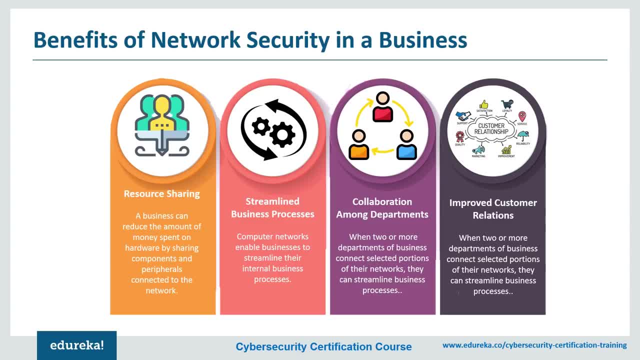 Second is a streamlined business process, which means computer networks enable businesses to streamline their internal business processes. third is a collaboration among departments. now, when two or more departments of business connect selected portions of their network, They can streamline business processes that normally take inordinate amounts of time. 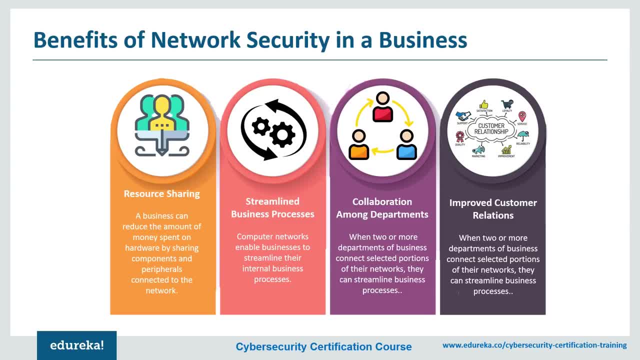 and effort and often poses difficulties for achieving high productivity. last but not the least is improved customer relations. network provide customers with many benefits, such as convenience in doing business, speedy service response and so on. There are many other business specific benefits that accrue from networking. such benefits have made it essential 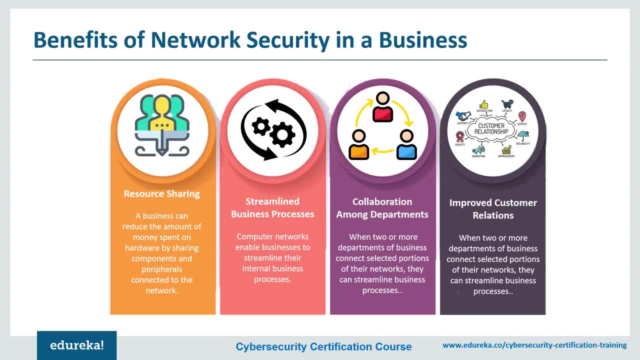 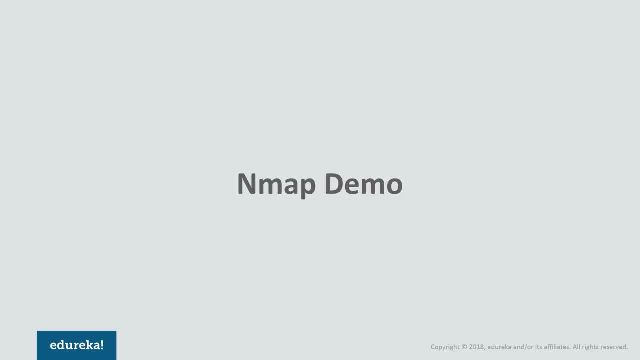 for all types of business to adopt computer networking and network security as a whole. Okay, guys, so now that we're done with the theory part of this tutorial, it's time we move on to the demonstration that I have in store for you, guys, today. 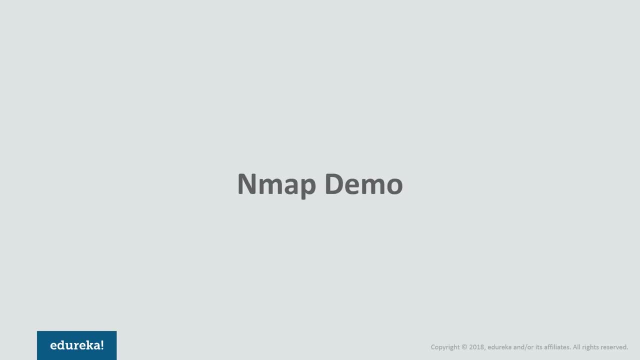 So for this demo we're going to explore a tool called nmap. now nmap is widely used in the cyber security industry for intelligence gathering before actually fixing any vulnerabilities that might be there in the system. So we're going to be actually seeing how we can use nmap. 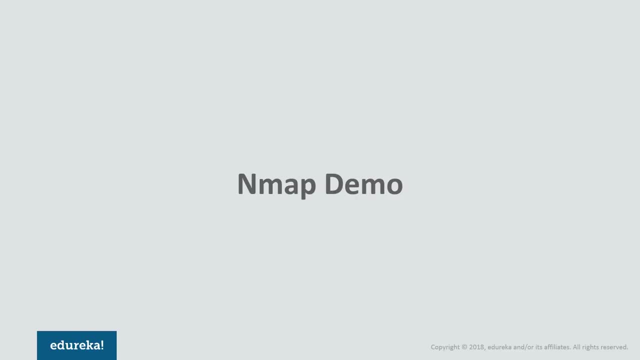 to get information about a server, then actually aggressively scan any subnet and a lot of port scanning and how you can actually write down all these scanned information into a file. So let's get started, So you guys can easily install nmap on your computers. 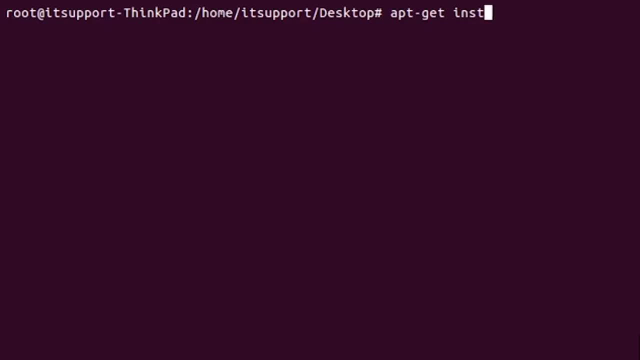 If you are running Linux by going apt, get, install and map. since it's already installed in my computer, I don't need to do anything. So, first of all, we're going to start out by getting information about any server that we want. So for this example, I'm going to be using edurekaco. 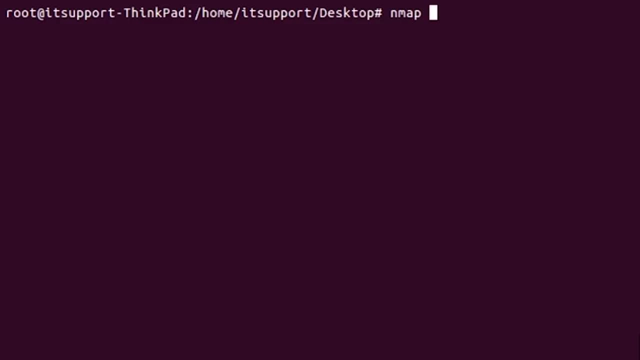 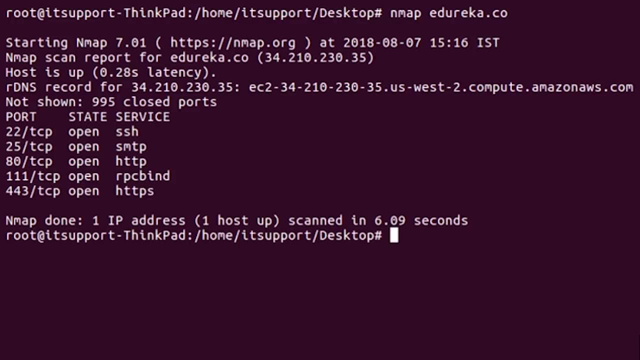 as the example server. So we go nmap space, edurekaco and it'll tell us a lot about the server. Let's see what happens. Okay, So, as you guys can see, it tells us all the services that are available on the server. 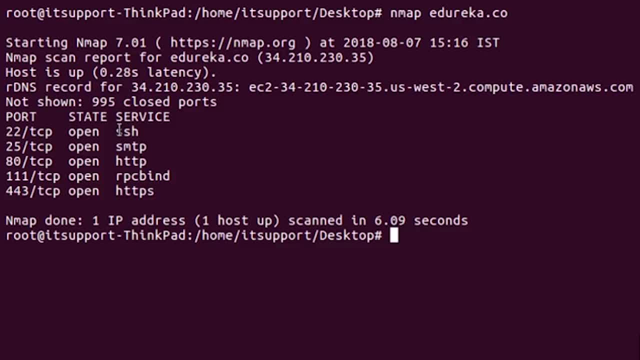 So we have an SSX server. that is SSX service, that is open and it also shows a state. so the states can be of four types. So one is open, one is closed, one is restricted and one is unrestricted. So open States mean that they are a place. 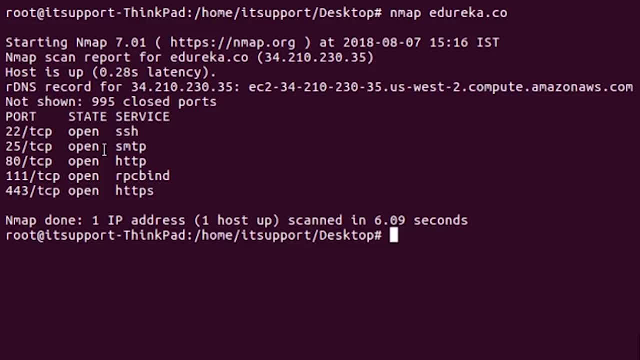 for a vulnerability to actually enter into your system. So when actually gathering intelligence, we are always looking for these open States. Okay, So for our next command we're going to see that how we can actually scan an IP address. So for that you can go nmap. 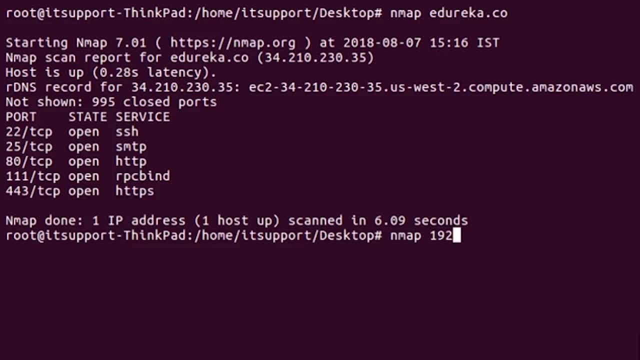 and then just simply type the IP address. That's one dot six dot one. So that's my gateway address. So it's going to tell us all about the Gateway. So yeah, and then map on our Gateway gave us a lot of information like what domain is open. 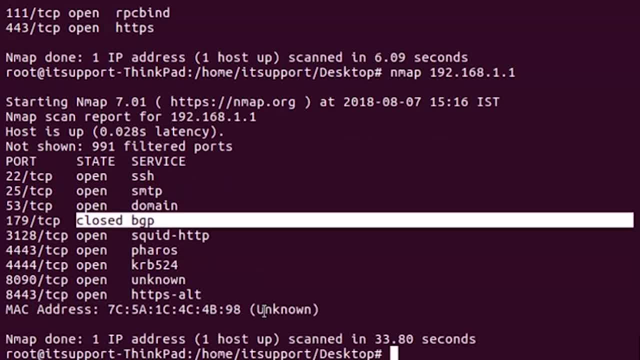 and so we can see that this BGP is closed. and so, moving on, we can also scan multiple IP addresses By actually spreading out the IP addresses with spaces 192.168.1.1, space 192.168.1.3, and you can run this. 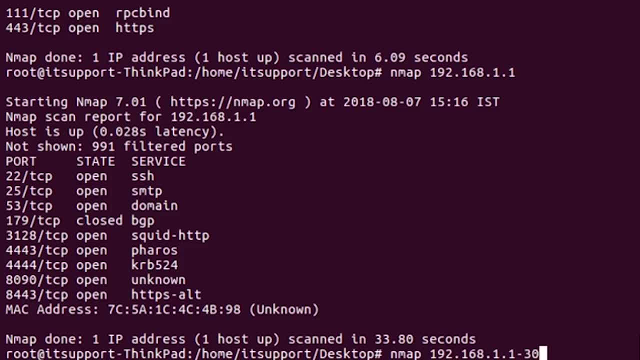 or you could just. if you wanted to go through 1 through 30, you could simply do this also. now I'm not going to run this command because this takes a lot of time, but it will always scan through 192.168.1 through 1 through 30. 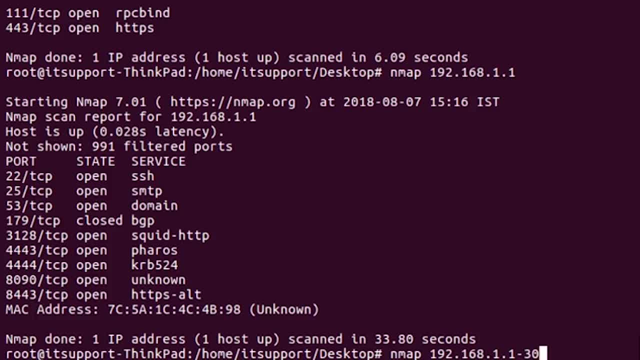 and will give you a result of all The 30 IP addresses. also, if you want to scan all 255 of them, you could just replace this with a star, And this is normally used when you are scanning your entire subnet, which is normally what you do as a network security analyst. 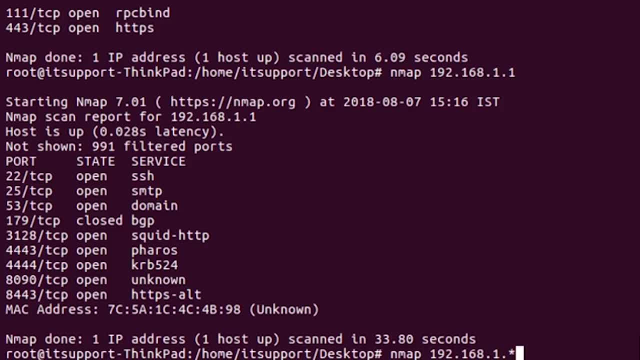 So this is what you would do, and you would just go out for a cup of coffee and then you would just come back for the results. It takes that much amount of time. So, moving on, we can also read a lot of information from text files. 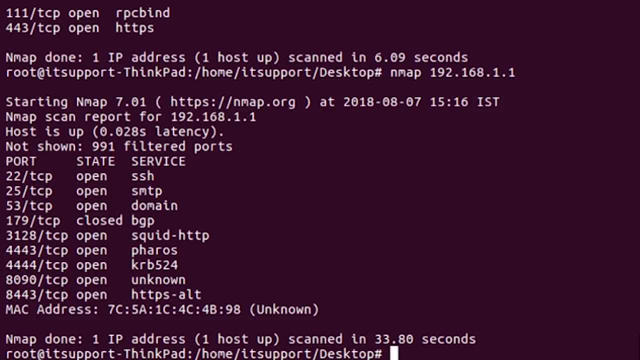 Like, suppose you have a few IP addresses saved on a text file. You can actually read them through nmap and scan them. So let's create a text file for this. touch targets TXT. So let's see if created that. we've created that. so 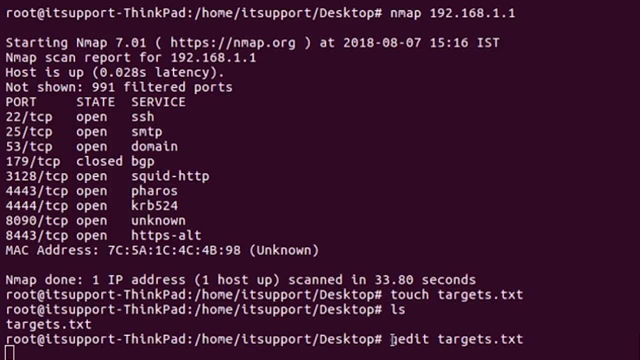 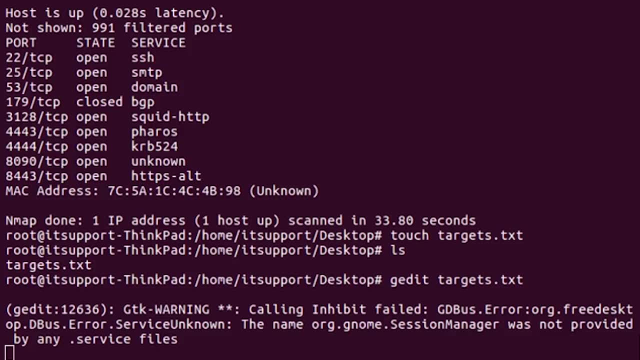 let's go get it. So let's give it two addresses on 192.168.3, like 1.15 and 192.168.3.. So let's give it two addresses on 192.168.3.4.. No, that sounds wrong. 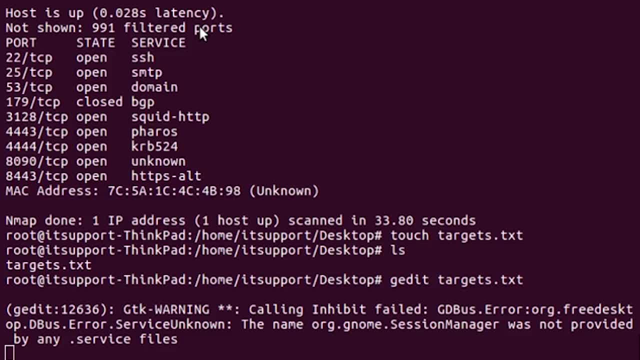 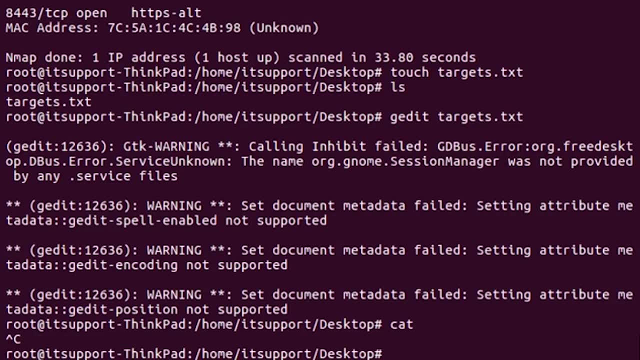 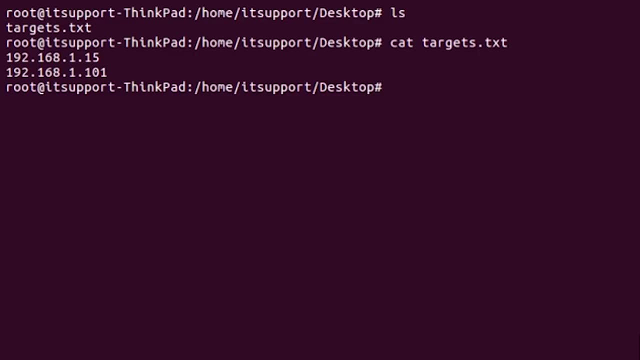 1.11.. Okay, so let's see if that worked properly. So we have our file ready with the IP addresses So we can simply read this with the IL flag. So you go hyphen I with capital L And then you just name your file. 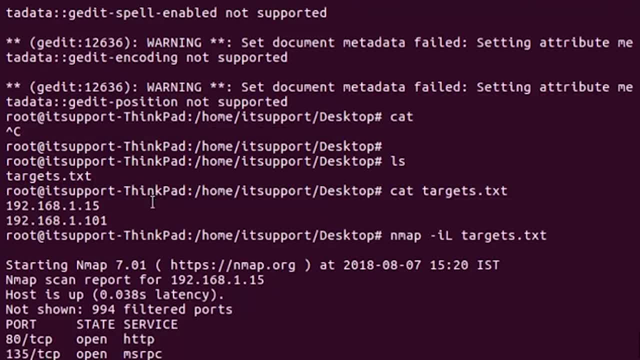 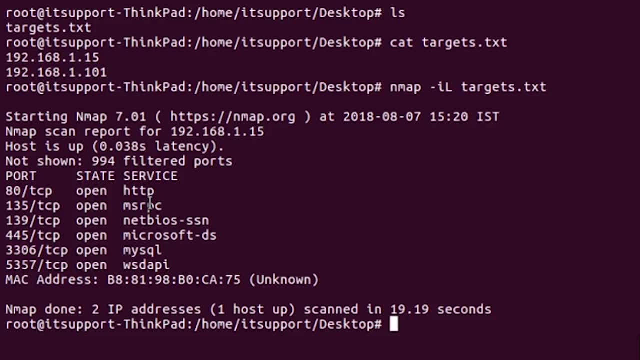 Okay, so, as you guys can see, it gave us information about these two IP addresses. Now moving on, and map can also be used for aggressively scanning an IP address. So for that you just go and map capital a and you name your domain. So at your record go. 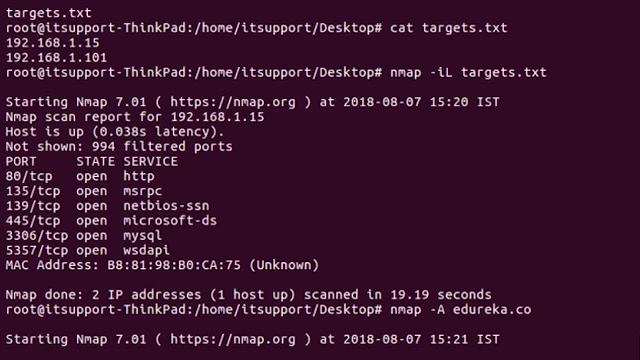 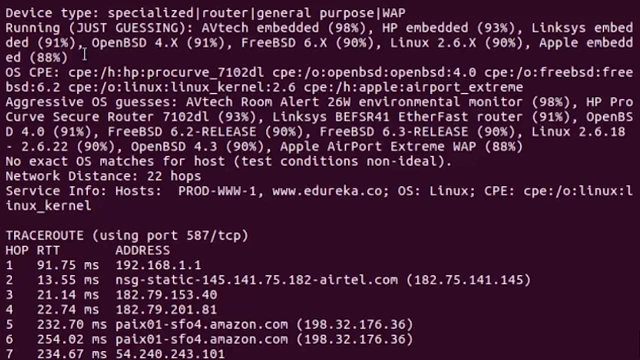 Now, an aggressive scan normally just means that it just gives you more information than a normal scan word Like it gives you the OS version and gives you the tracer out and it'll give us a lot more information about certificates and stuff. Yeah, so you guys can see, we've got the tracer out. 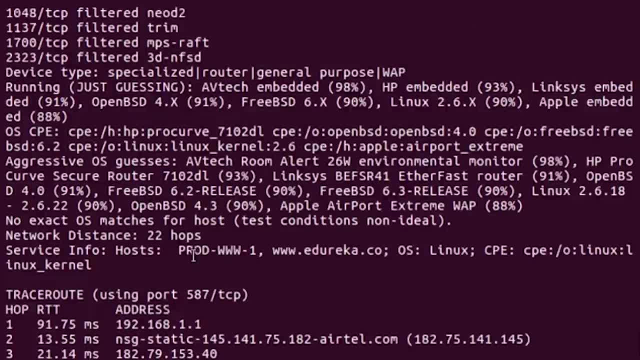 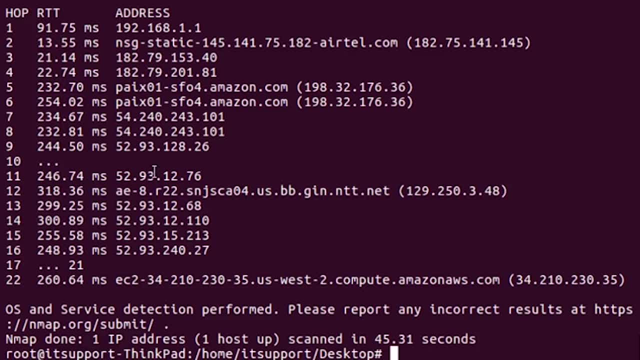 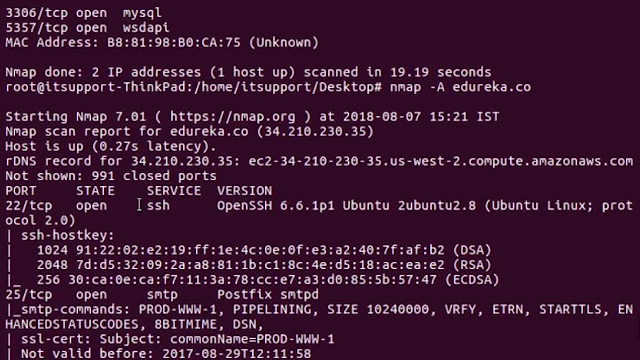 for the dress. So give you the entire way. The router has actually routed the packet to, from your client device to the server device, and it also tells us which ports are open and a lot of other information is given about the server out here. Now, sometimes you also want to know about the OS. 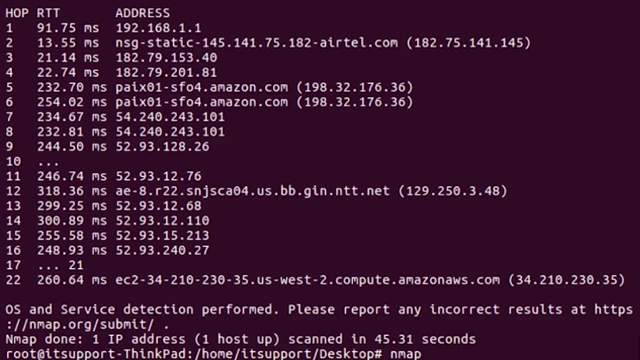 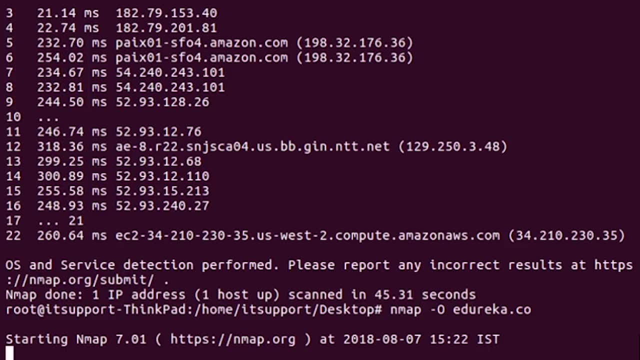 that the vulnerability system is running. so you can go and map O and edureka Go and that will give you an information about the operating system being run on that So. so, for example, edureka will have a Linux or running on the system and that will be easily shown by nmap. 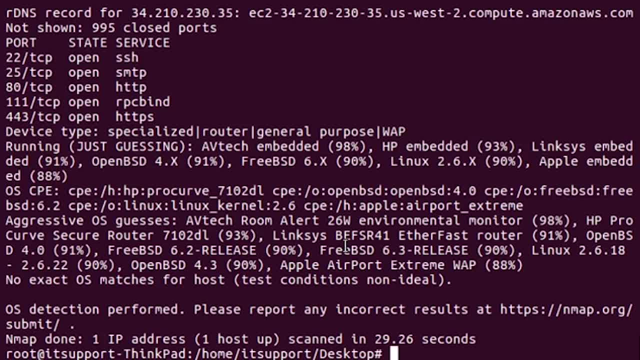 So, as you guys can see, it gives us a lot of guesses about the OS is that could be on it. So nmap can never Surely tell which OS is running. It'll tell you a guess. So whichever guess is the most accurate will be the one. 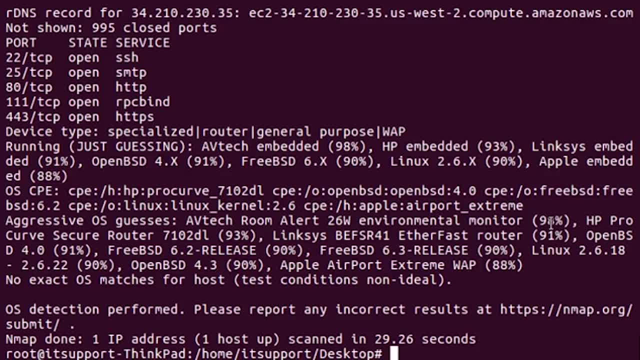 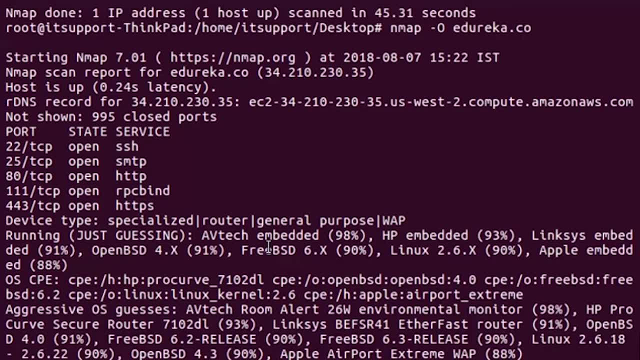 so it's like this: after a groom alert, 26w environmental monitor is running, that's a 98%. Yes, and that's free curve. secure router is also there, which is a 93%, and you can get a lot of information about the OS and like out here that we come to know. 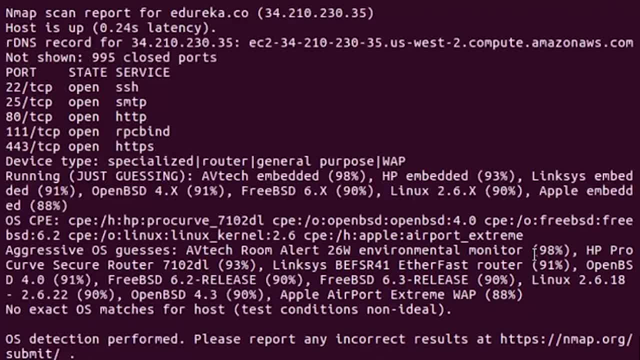 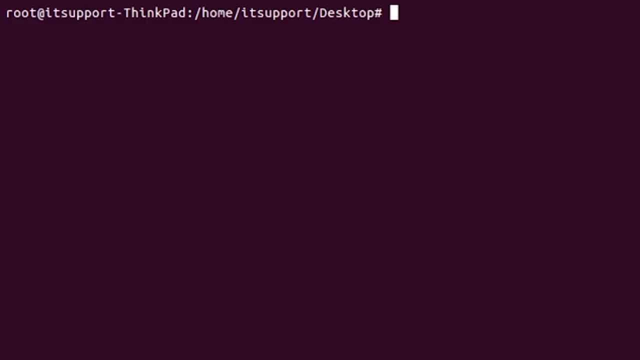 that it's a Linux 2.6.. Point two to OS that is running on there. So sometimes, while gathering intelligence before penetration testing, y'all might want to know what route a packet takes from your computer to the server You're actually communicating with. so for that you go nmap hyphen. 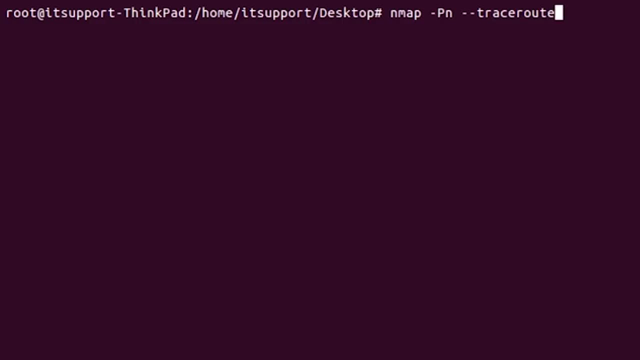 capital, P and hyphen, hyphen, trace route and the name of the domain. So for an us, edureka Go. So this will tell us how many hops there are in reaching the edureka Go servers and the Most of IP addresses that we are going to go through. 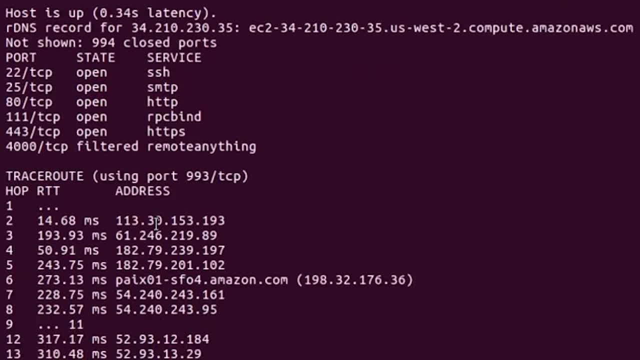 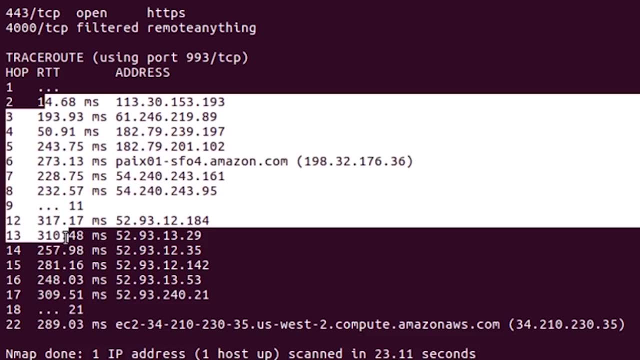 So, as you guys can see, it told us entire hop route. We have 22 hops, So these are the dresses that we went through and this is the route and the ping at each address. So sometimes also you all might want to know about the service version. 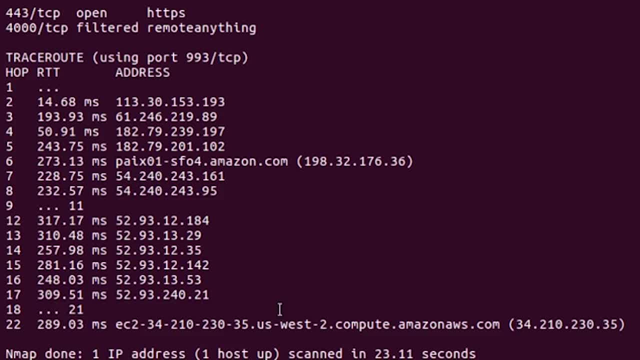 So suppose there's an SSX service open and you want to test it for vulnerabilities. So it's always great to know the service version. So for that you go and map hyphen s and capital V, which stands for service version, and you can run this entire command on a solo. 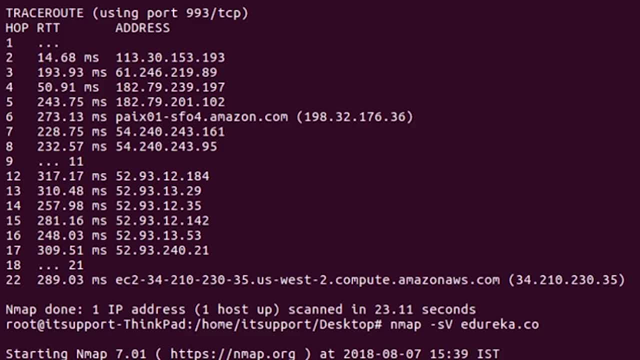 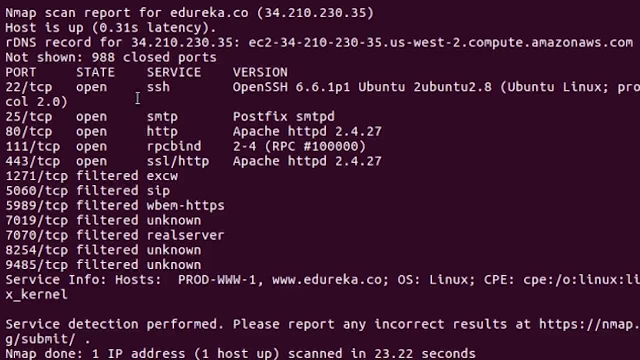 So, like previously, it gave us the state and the name of the service. Now it'll also give us a version number. So, as you guys can see, it tells us the SSH version is open- SSX 6.6. One. and told us the SMTP is post-fix: SMTP D. 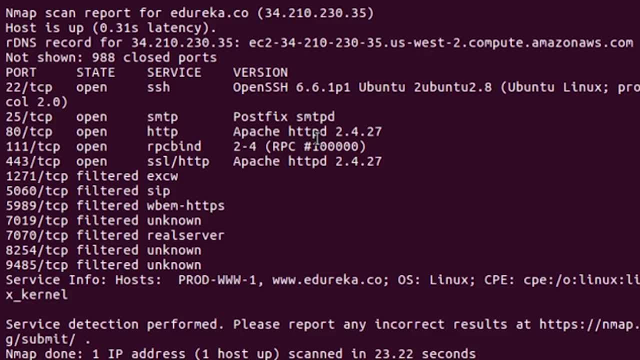 Our HTTP is an Apache HTTP D server with two point four, point two, point seven, and yeah, that's about it. So nmap also allows you to scan port numbers. so you can scan port numbers with the P flag. So next you just have to enter the port numbers you want to scan. 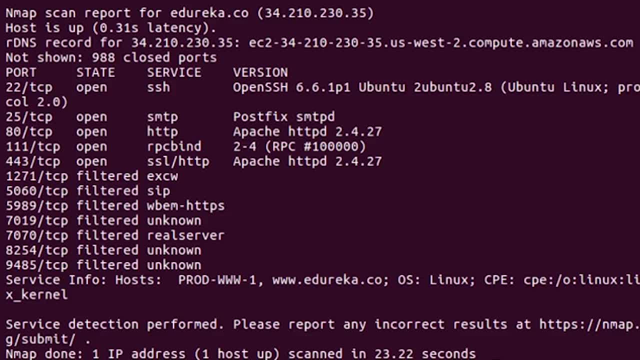 So suppose you want to scan through 20 to 25 and you can also scan multiple port numbers by separating them with commas, So you go 80 and which is basically HTTP, and suppose you want to go through one one one, which is the RPC bind. 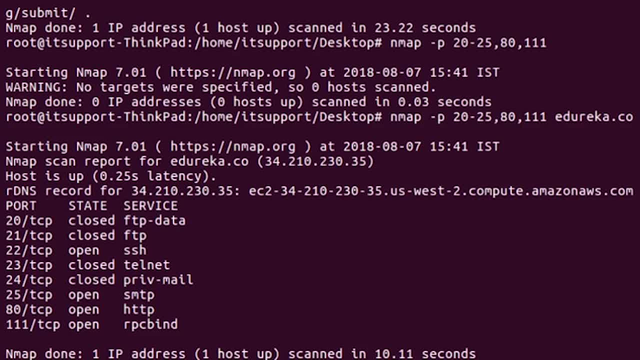 So you can scan these port numbers. So it told us the information about 20 to 25. like we can see that the FTP is closed, So it should be closed with. the FTP is really easy to hack into and the others are open, So that's, that's not a problem for us. 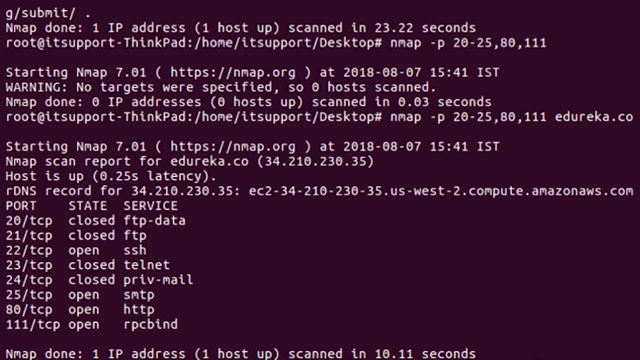 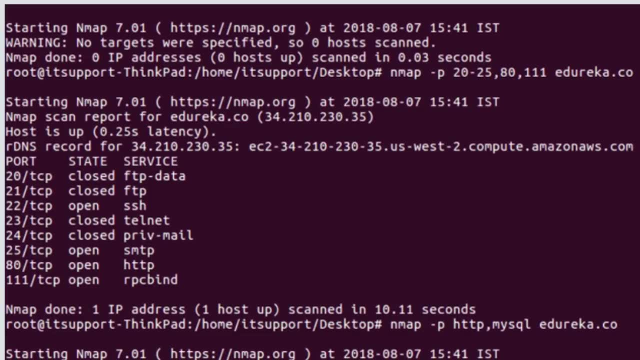 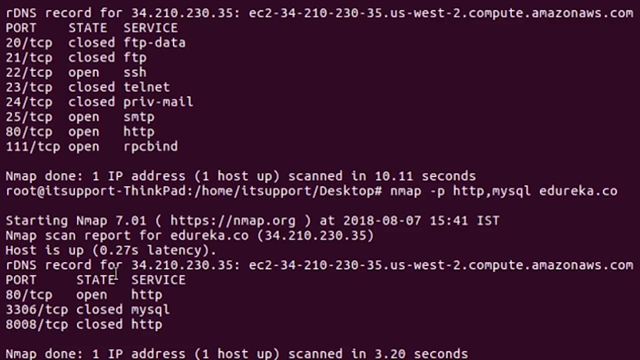 So we can also scan port numbers by their name. So we want to scan the HTTP port. we can go and map hyphen P, HTTP. We can scan for a mysql port, So let's try it out. So, as we see, our HTTP port is closed and it's running on 8008. 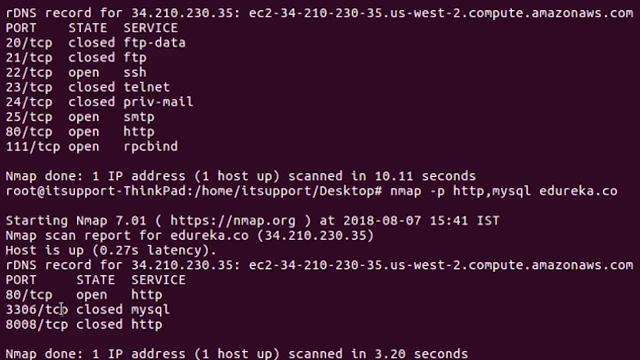 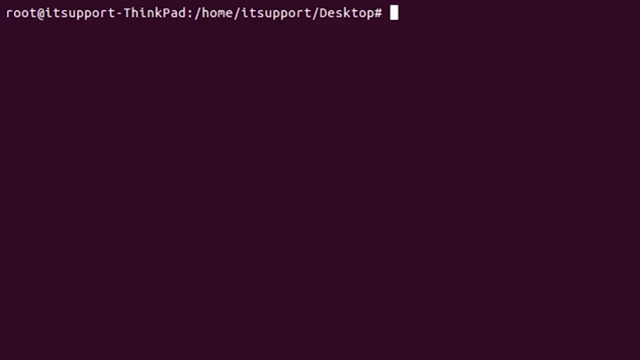 and there's one running on a port number 80. There's also a closed mysql service running on port number 3306.. So that's a lot of port numbers. So sometimes you all also might want to save the results of your scan into a text file. so you can easily do that by going nmap. 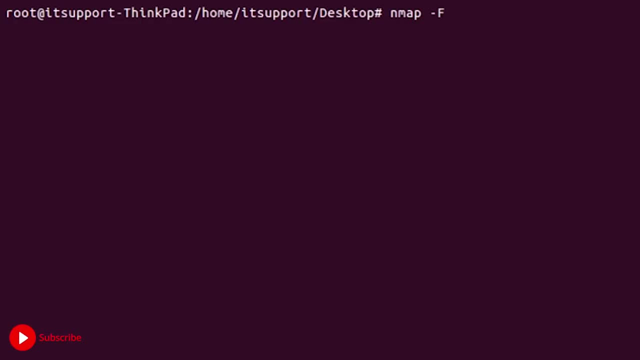 hyphen F. So F will actually do a very fast scan. and then you use the o n flag, small o and capital N, which tells us that we're going to write it down into a normal text file. So we're going to do it. logs dot txt. 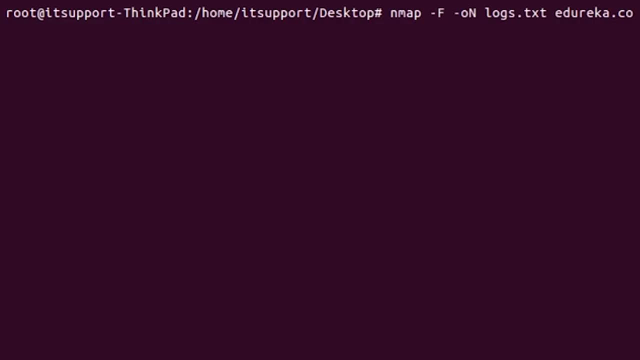 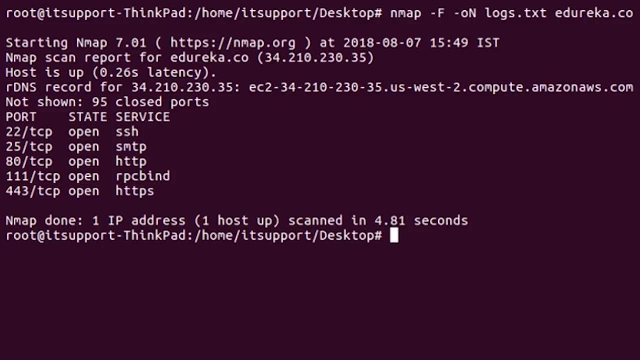 and we're going to scan through edurekagov again. So let's see, So our scan is over and, as you guys notice, that was a very, very fast scan and if we go into our directory we see That we have a logs or txt file. 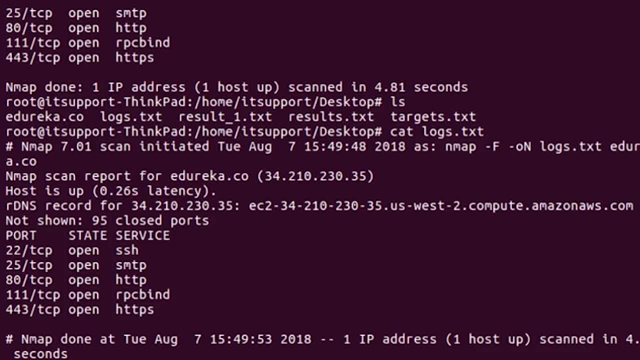 and if we got that file, we see it's the same output. So we've actually written down a file with all the scan results. So that was it for an nmap demo. guys, I hope you all learned something valuable today, And that's it for this video on network security tutorial. 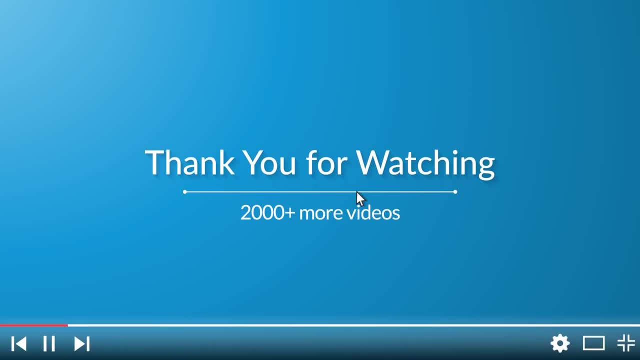 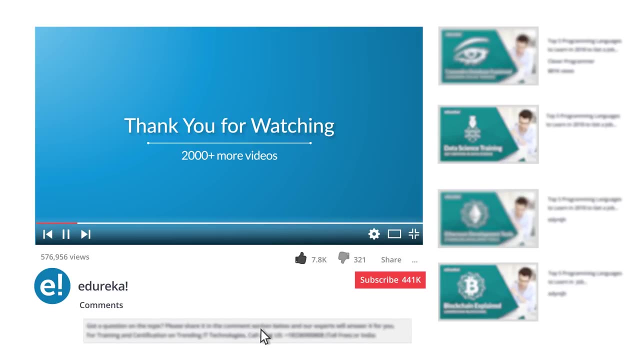 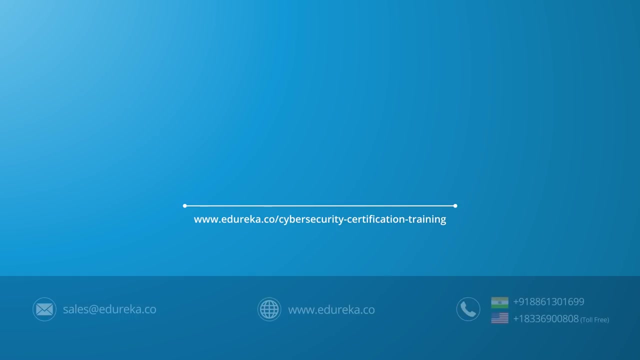 Goodbye. I hope you have enjoyed listening to this video. Please be kind enough to like it and you can comment any of your doubts and queries and we will reply By them at the earliest. do look out for more videos in our playlist and subscribe to edureka channel to learn more. Happy learning.